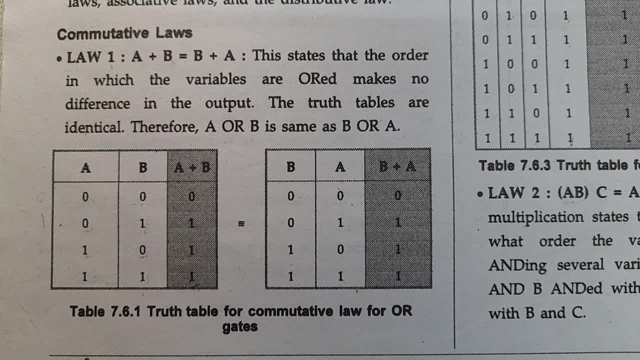 b. it has a plus b, capital b, So a plus b can be a plus a or r plus a, So an Los retos ab and an Los retos b are variables. okay, When we say plus b, it represents the odd. 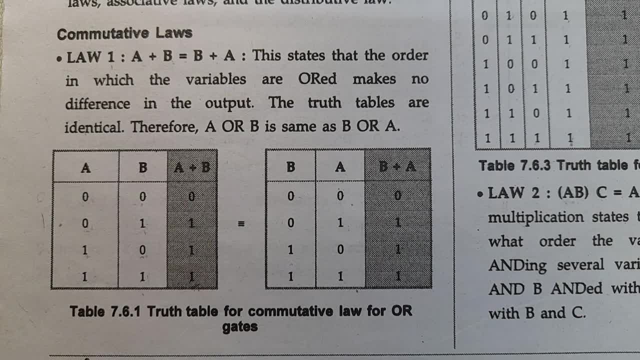 operation, All the opportunistic operations like that are all R, So also the result. e está similar with LHS, only a plus b equal to a. So what will be the result? in a LHS, the same as th e in RHS, l also. So no matter, which is a plus b, is an Or it won't be the same, So this is commutative. Now it is the first law of sunk a and the result is full of double a. this, Kevin, As you can see the couplet, This one and the revolution by LHS a plus a. So it is same. in a LHS an Lo Well, in which the different McLwans used the 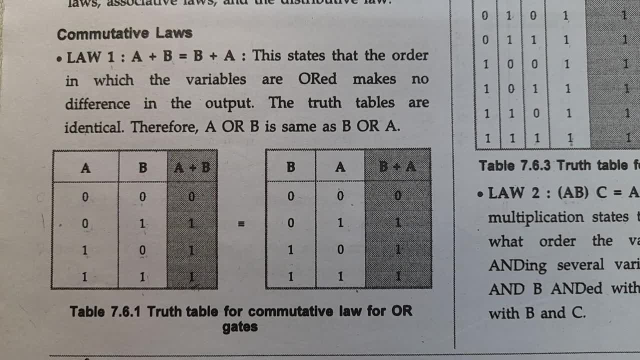 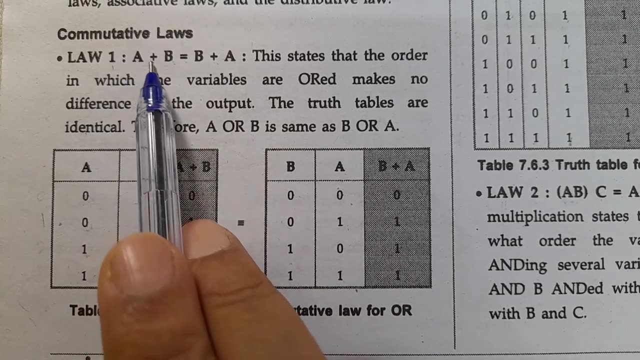 Variables are odd makes no difference in the output. The truth tables are identical. Therefore, A or B is the same as B or A. Here plus is there. we have to read the plus sign as R, A or B Equal is the same as B or A. 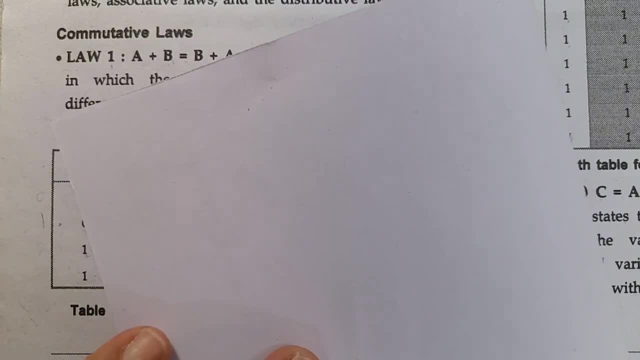 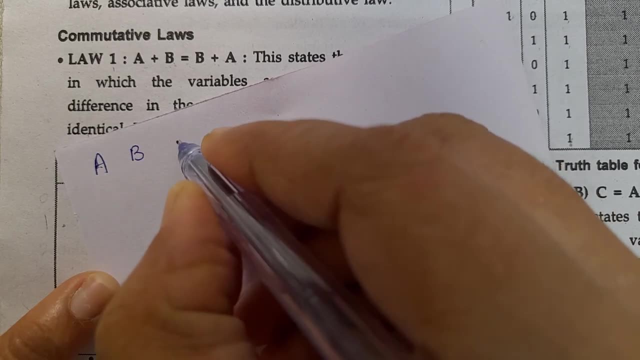 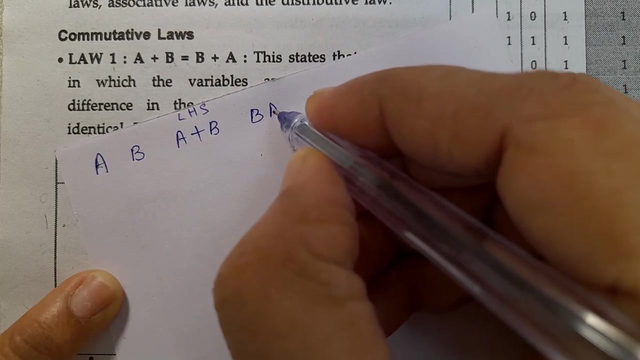 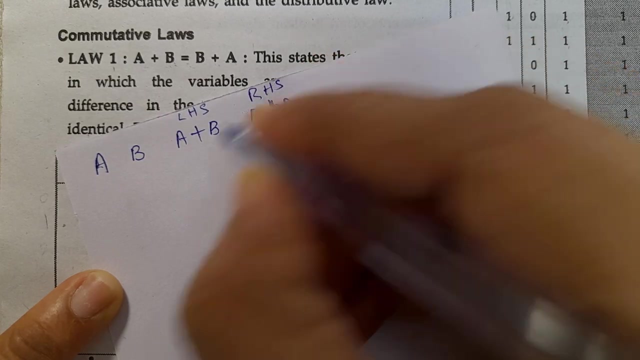 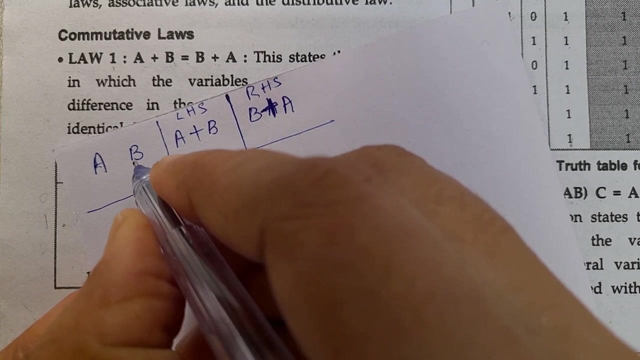 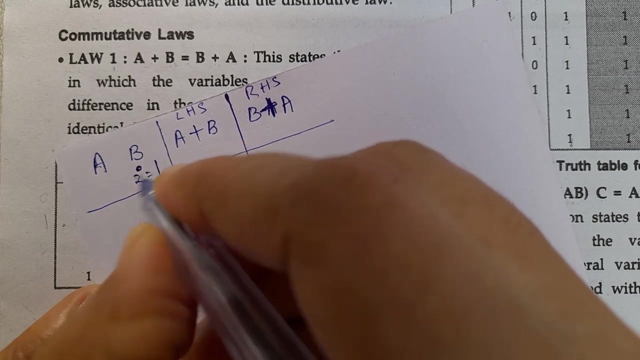 So how to write the truth? table first: A plus B. So A, B are variables. So A plus B, this is for LHS. RHS is B plus A, This is for RHS. So here take the binary input. So 2 power of 0, 2 power of 0 is 1. 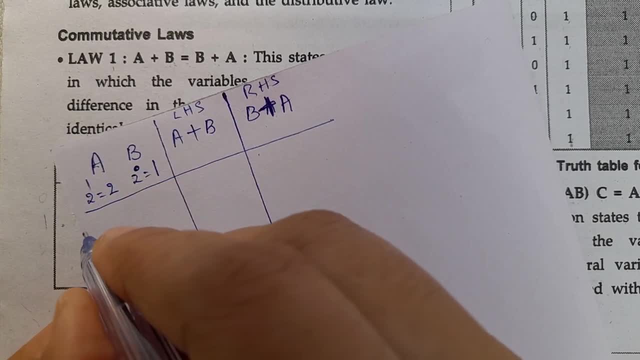 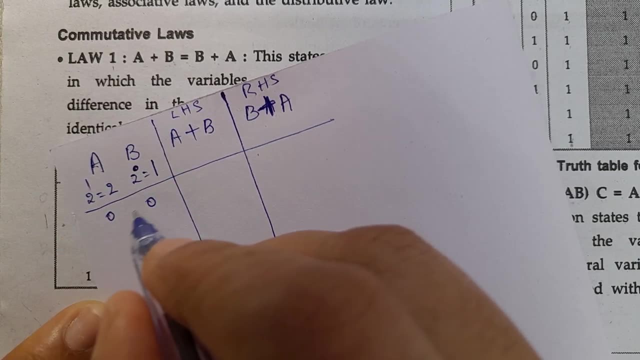 Next, 2. power of 1 is 2. First, 0,. 0 means both the inputs are 0. A, B are variables. So if we say 0, both the inputs are 0, So then what about A plus B, A or B? 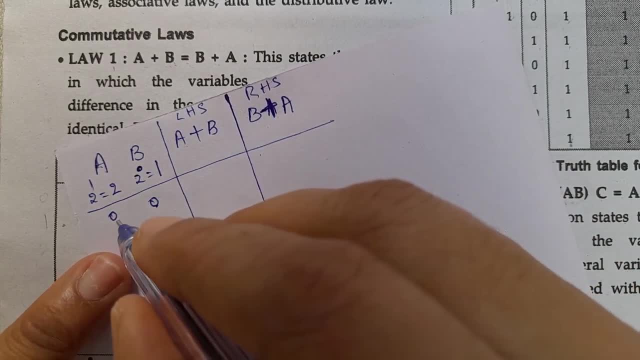 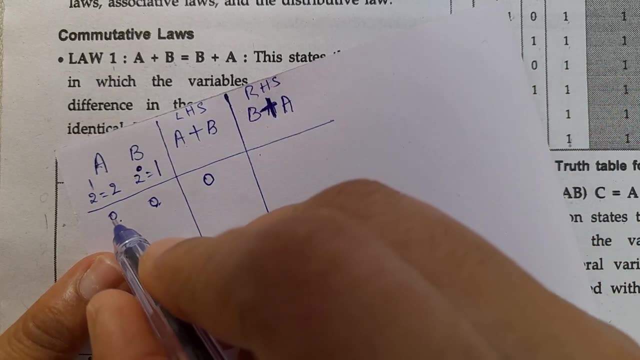 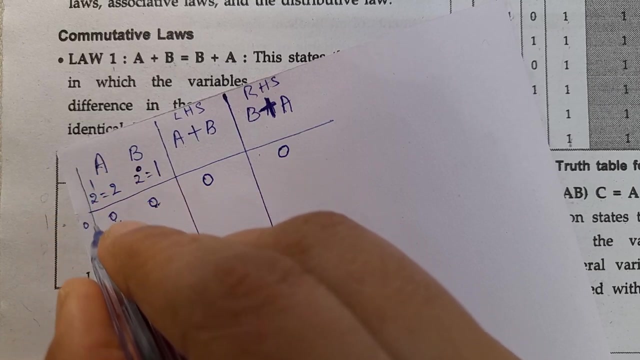 If we say R, we have to add 2: 0 plus B is 0. 0 plus 0 is 0. Next B or A. B or A. 0 plus 0 is 0. Next 1. Here: 0 is 0. Next is 1. 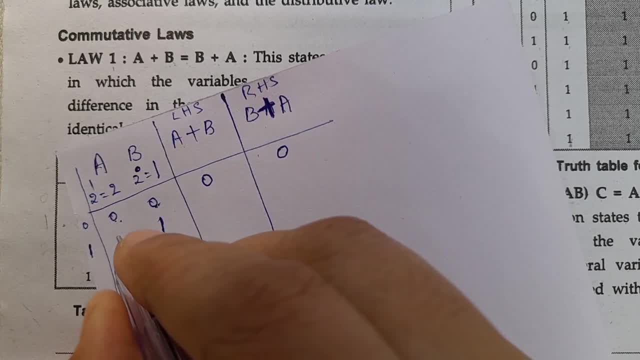 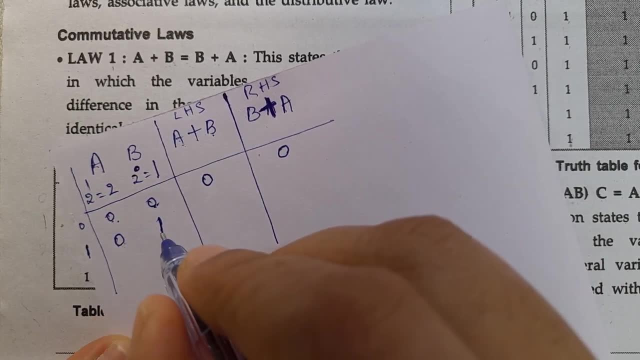 1 means this should be on, So B input should be on, A input should be off. So if we say A plus B, A or B: A is 0 plus 1, so that is 1 B or A. 0 means 1 plus 0. 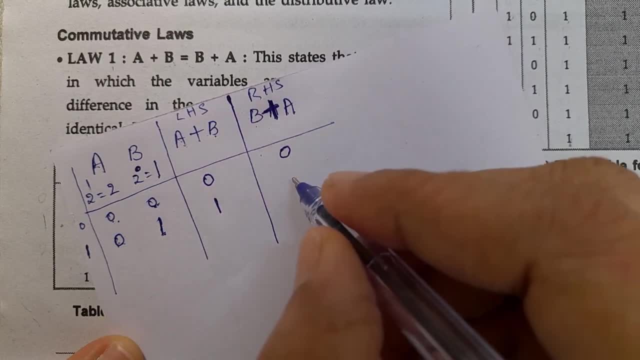 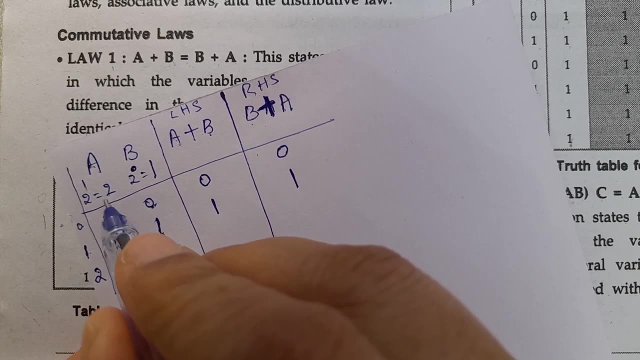 B is 1. 1 plus 0 is 1. Next 0 is 1, so that is 2. 2 means this one. This should be on, A is on, B should be off. So A or B, A or B. 1 plus 0 is 1. 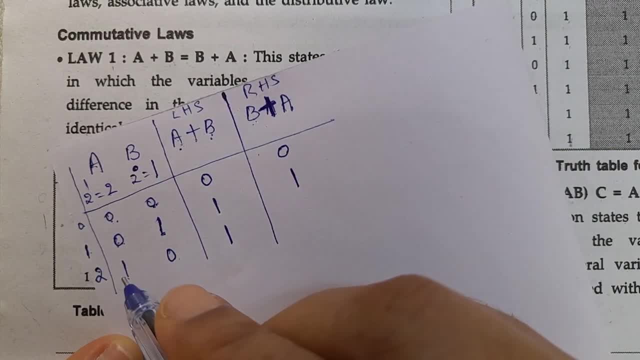 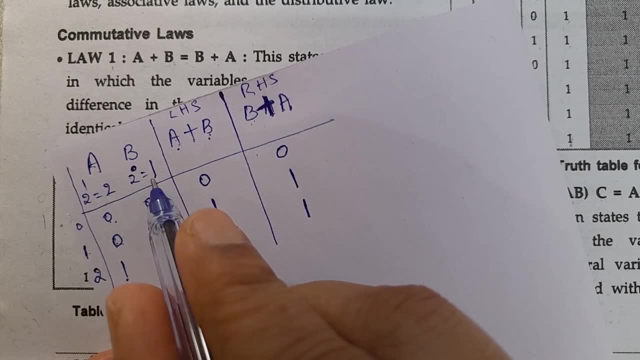 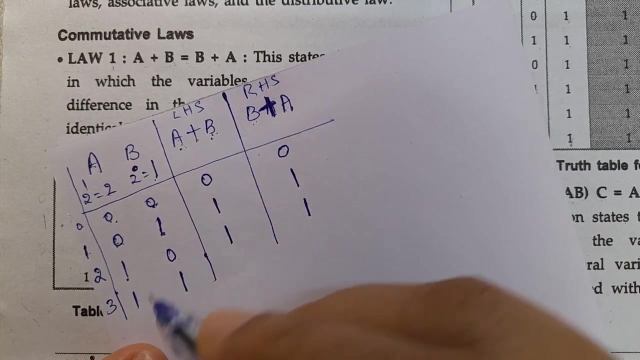 B or A. 0 plus 1 is 1, Next 3. 3 means 2 plus 1 is 3, So both the inputs should be on. So then A or B. So 1 plus 1 is 2. 2 means 1, 0. 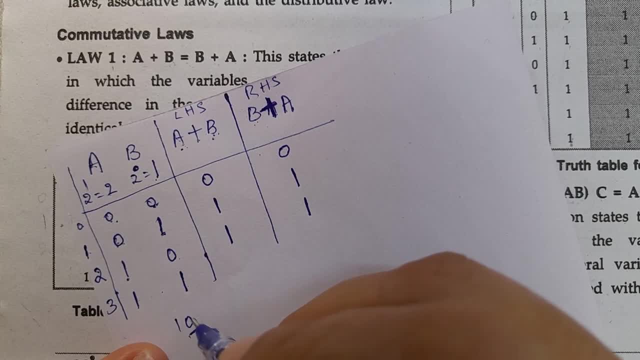 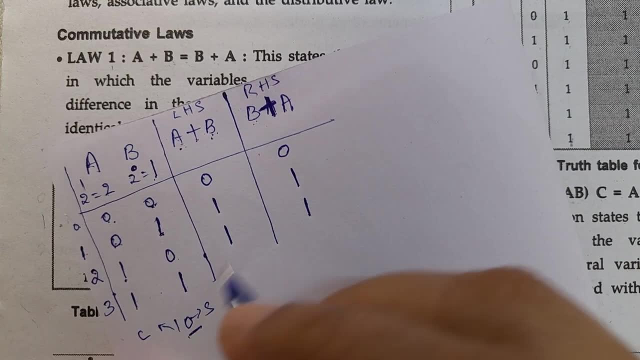 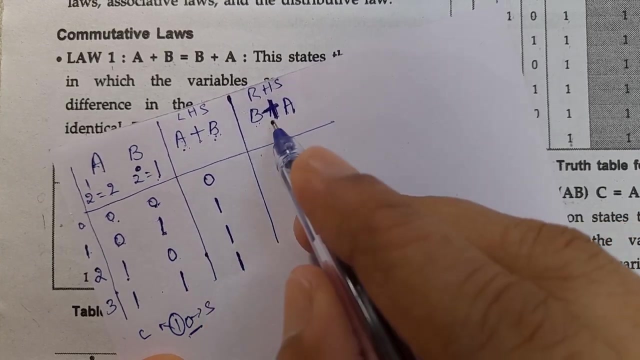 1, 0 means LHS bit, So we are considering the sum, So we are considering the carry of the highest significant bit. But what we have to take here is 1 is the result. So 1, B plus A, B or A, So 1 plus 1 is 2. 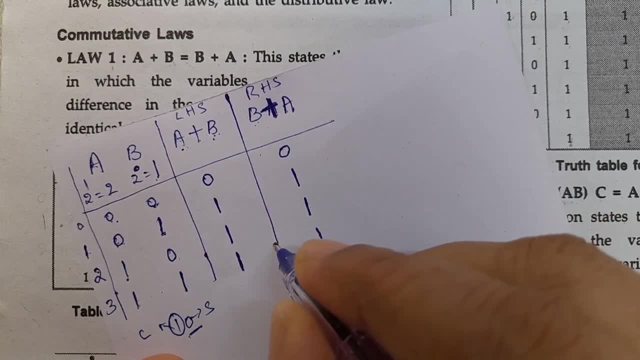 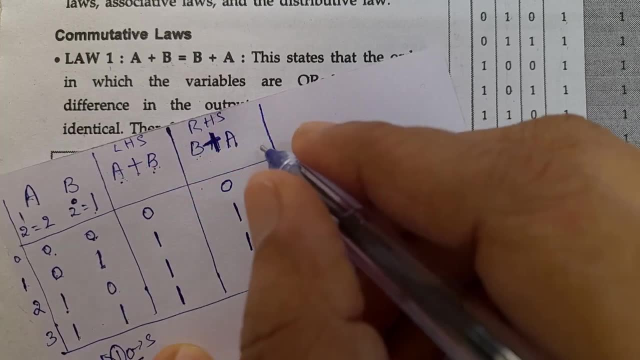 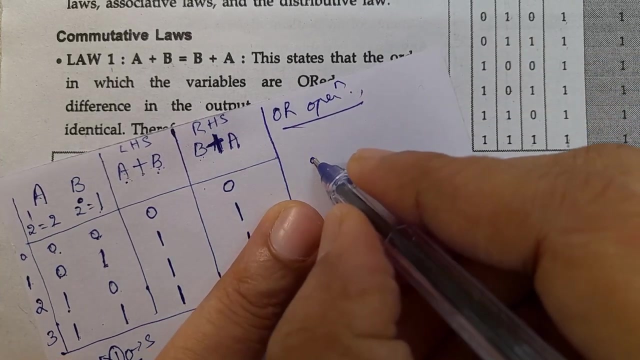 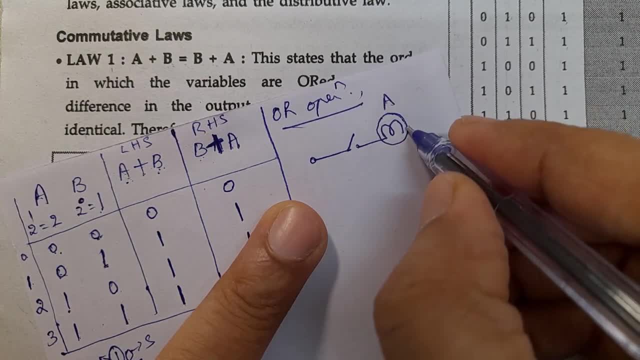 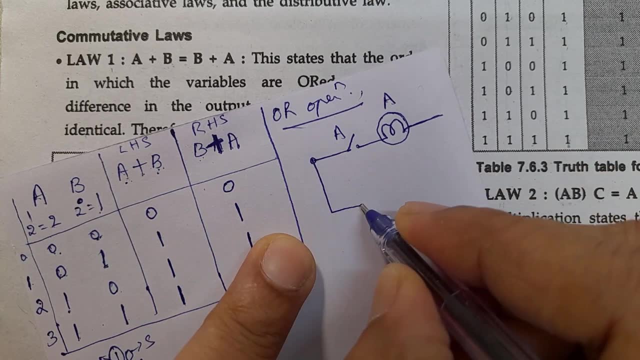 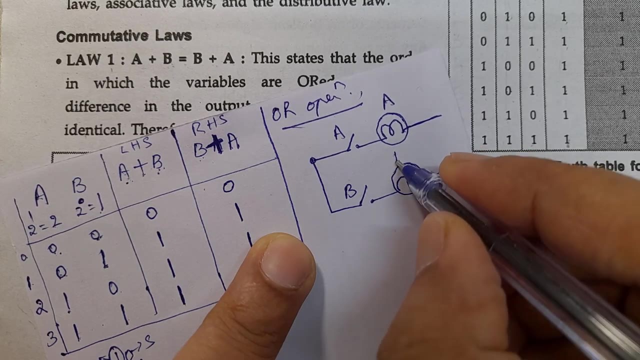 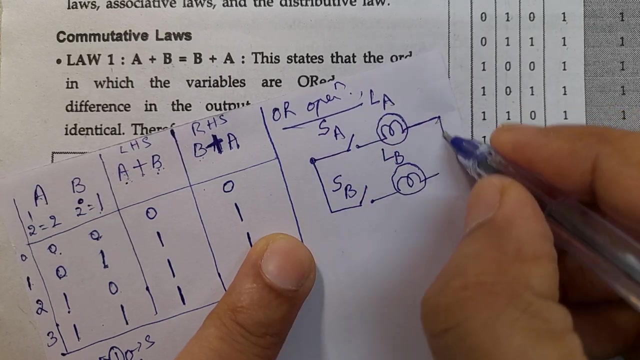 So this I call it as A bulb, See So switch A, This is A switch. Next, This is for B switch And also B bulb. This is for Lamp LA Lamp LB Switch, SA Switch, SB. Ok, These two are parallel connection, So here AC input is applied. 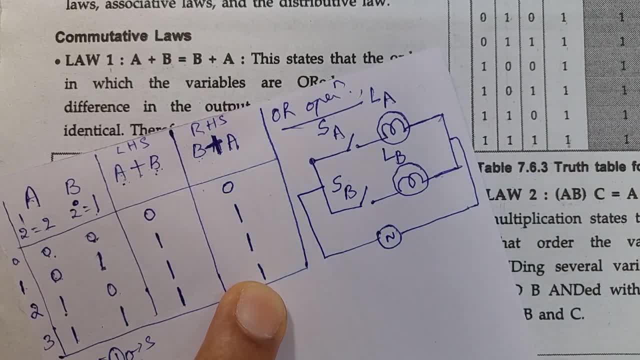 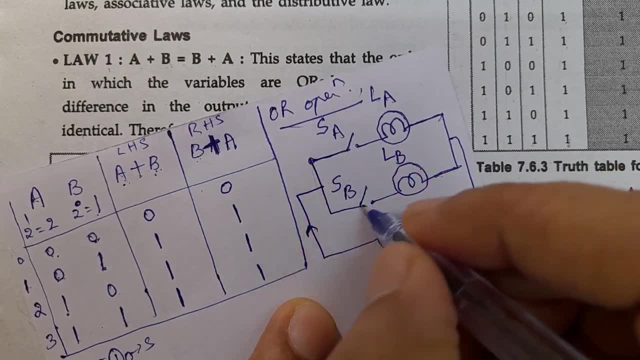 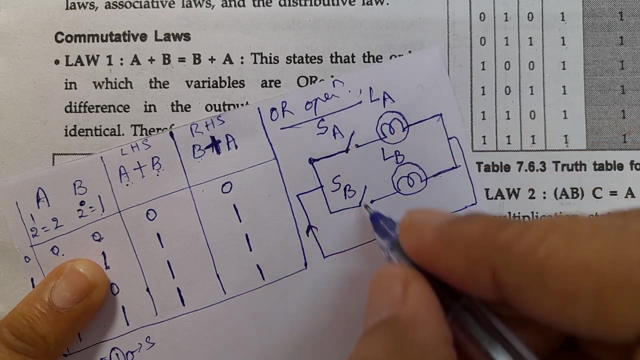 It is alternating current. This is what it is After AC is applied, AC supply is applied, AC current is flowing. So here it is. So here it is divided. Current is divided. These switches: See A switch: It's open. Open means 0. B switch is also open. 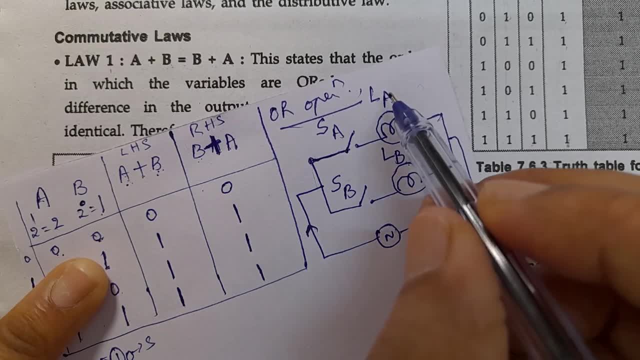 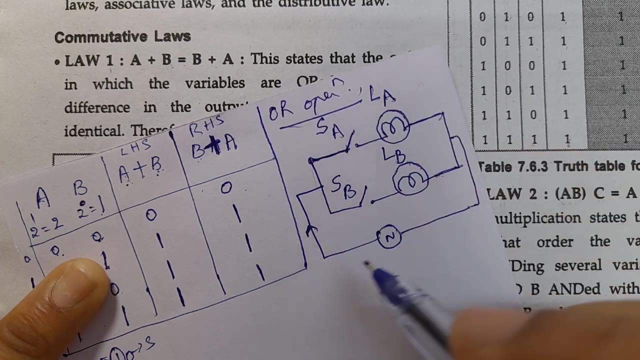 Zero. So A or B Or B or A. What happens? It becomes zero. Which switches also can be turned on? One, Two switches are there. There are two bulbs. A switch is not on, B switch is not on, so room is dark, so darkness is there. so 0, 0. 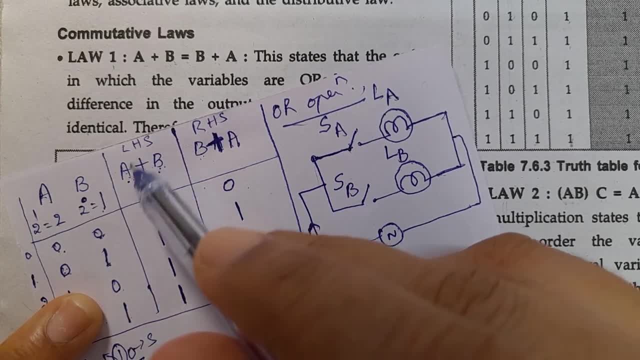 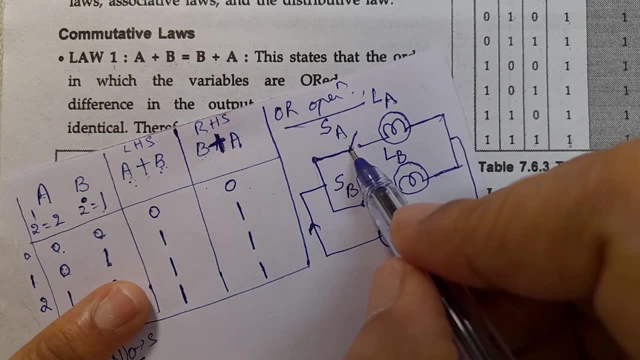 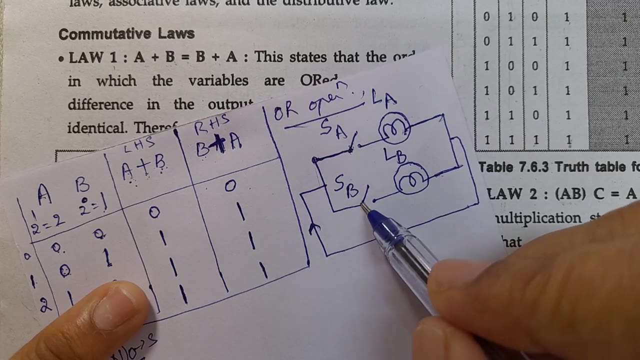 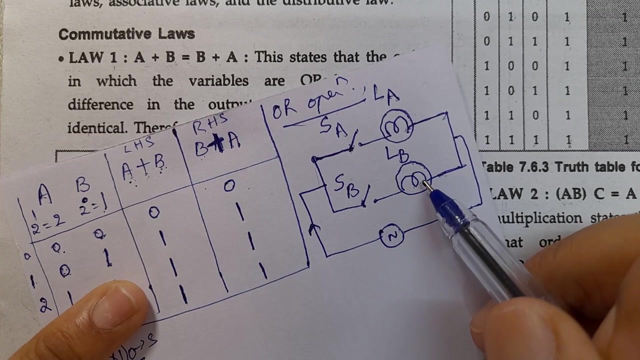 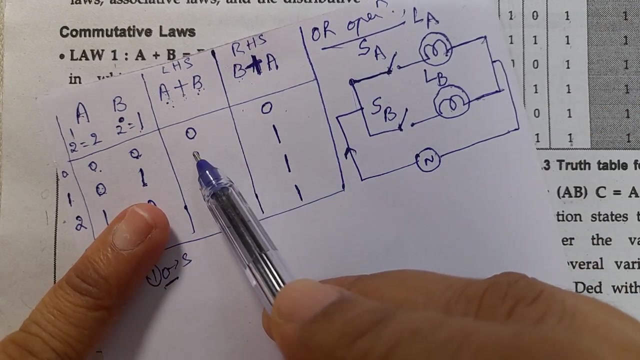 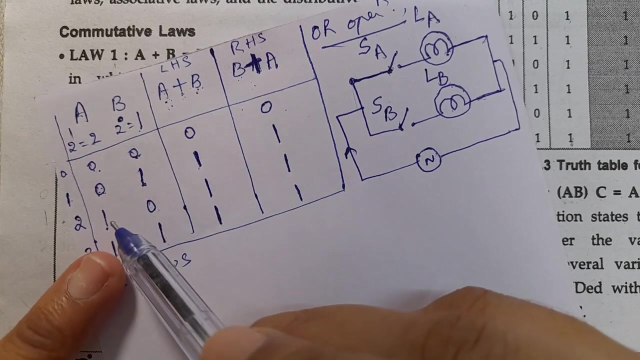 Now A plus B. A plus means OR operation. now A switch is off, B switch is on. but if A switch is off, lamp will not glow. so light is off, bulb is not glowing. But if B switch is on, bulb LB bulb is not there, lamp B is glowing. there is light in room. so A or B is on. there is room A or B, or B or A is not there. this is one room. there is light in room. A is on. I have closed this switch. 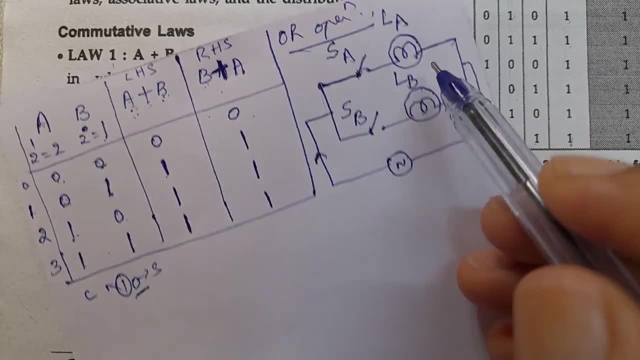 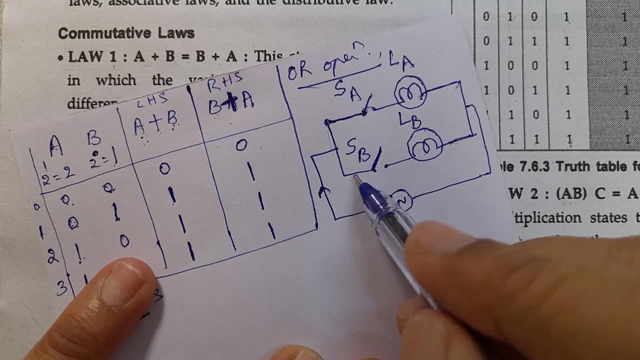 If I close bulb, where is the lamp? This will glow. see now, switch B is off. if it is off, it is open. so there is no current flow here. so what happens to bulb if it is off? what is the current flow? 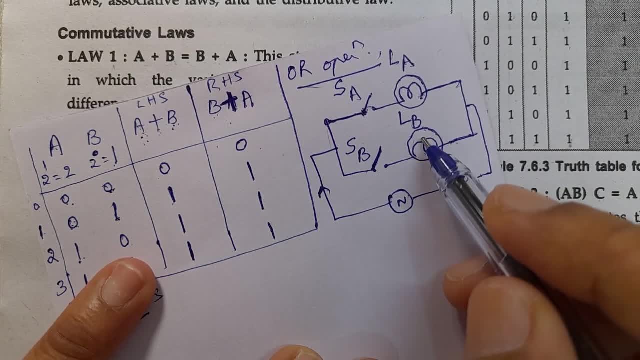 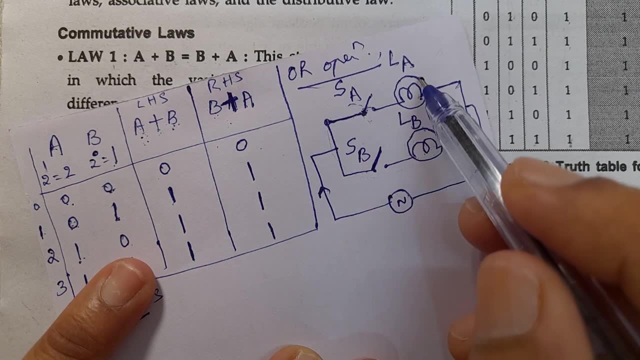 Bulb does not glow. it is not glowing, so there is light in room because A switch is closed. see, A switch is closed. so where is the lamp? where is the light? it is glowing, So this room switch is on and off. 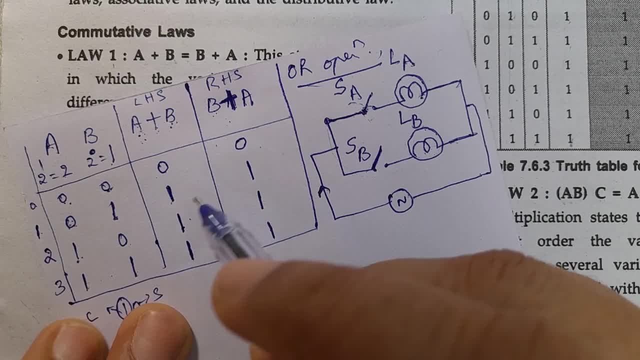 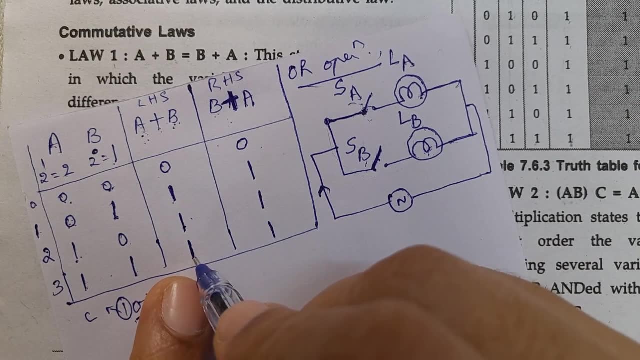 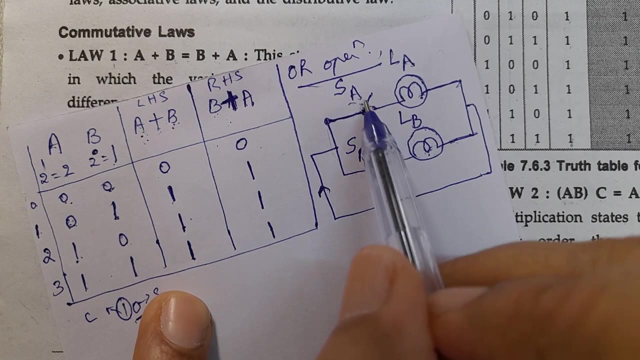 That means there is light in room. so I will turn on both the switches. so both the bulbs are glowing, so there is light in room. now If you turn on any of the switches, if you turn on any one switch, there will be light in room. 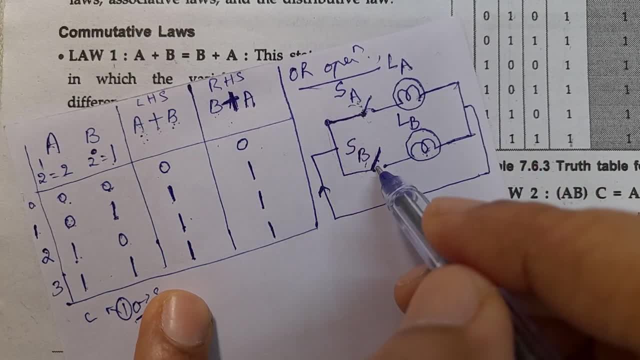 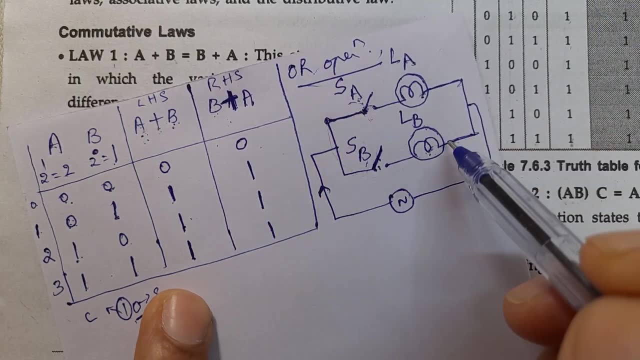 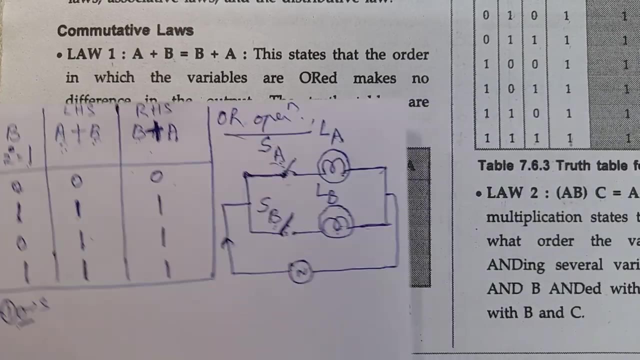 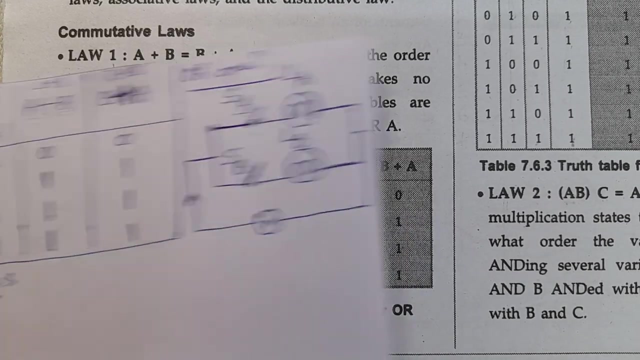 So this is parallel connection. So both are off means there is darkness in room. So this is for parallel connection or operation: See here. So this is correct 0111, here B or A is 0111.. 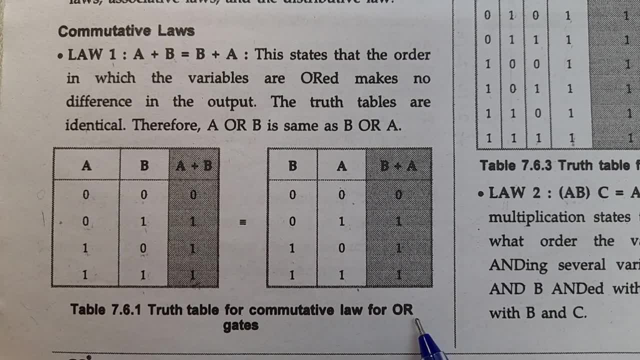 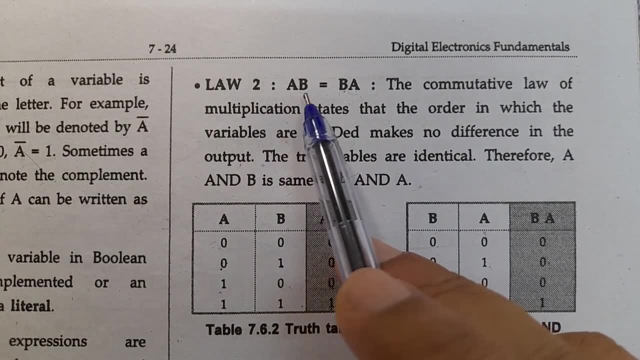 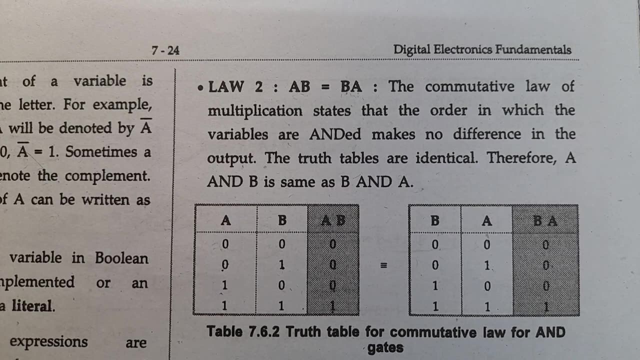 So this table, 7.6.1, truth table for commutative law for OR gates, Next law: 2.. So AB equal to BA. Here multiplication is done. The multiplication is called AND gate. So we multiply AND gate only. 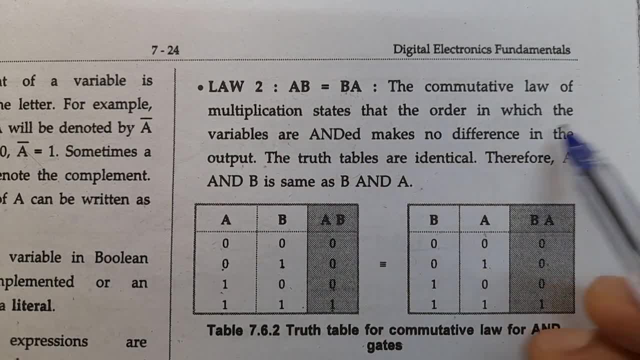 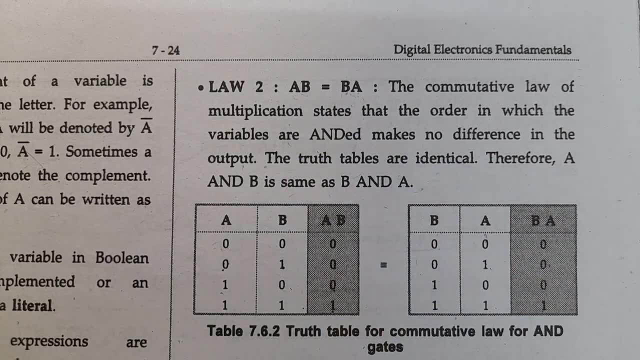 The commutative law of multiplication states that the order in which the variables are ANDed makes no difference in the output. So AND operation is same, The normal multiplication A is the same, So here ANDed makes no difference in the output. 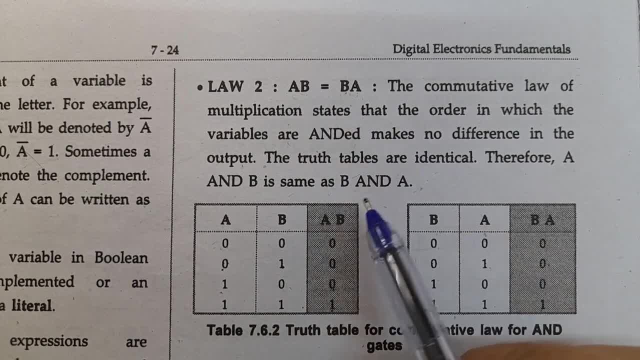 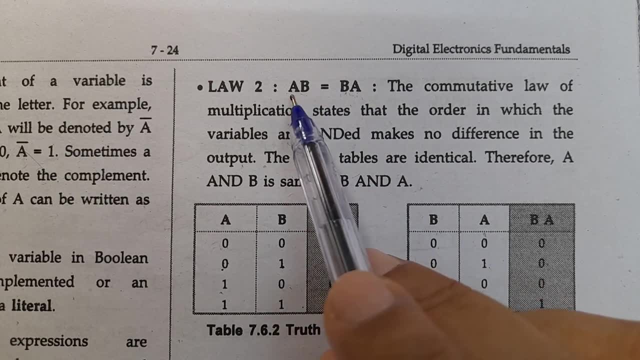 So there is no difference in the output. The truth tables are identical. Therefore, A and B is same as B and A. Now we have to read here, We should not read AB- A and B is same as B and A. 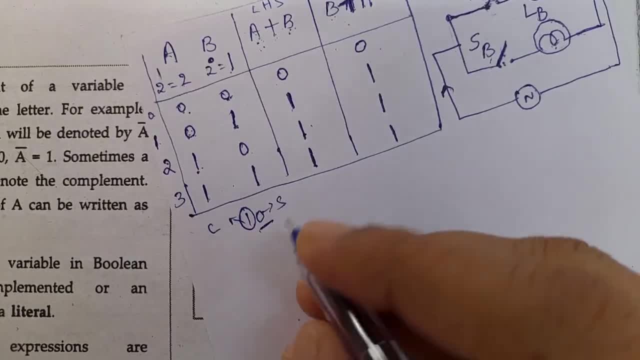 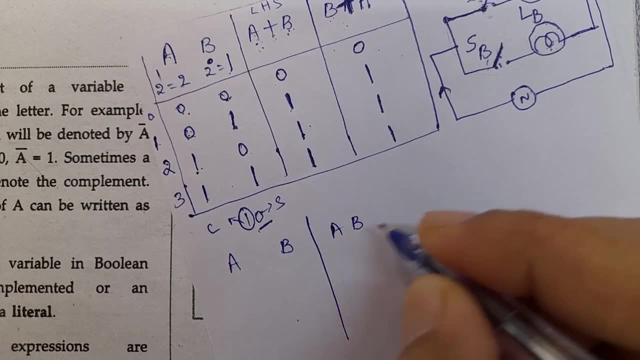 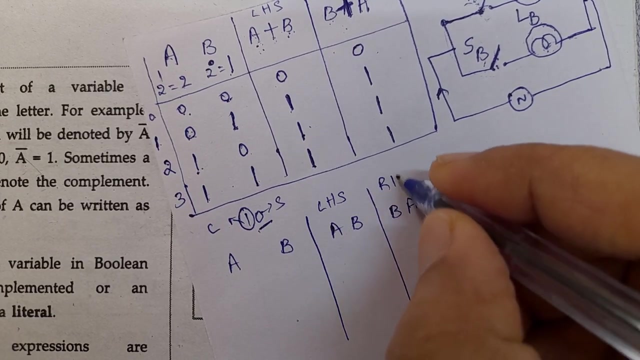 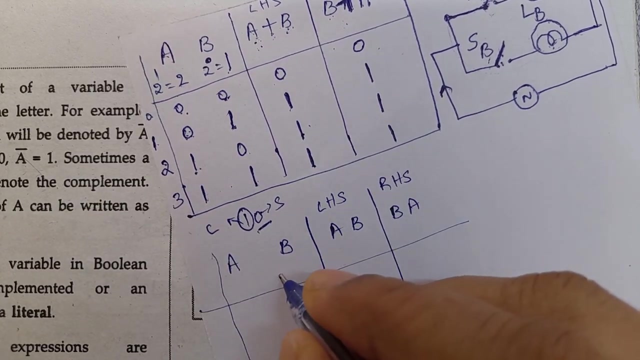 This is the truth table. So AB are inputs A and B. This is for LHS. RHS is B and A RHS Is it? both are same or not. We have to check it. So 2 power of 0 means 1.. 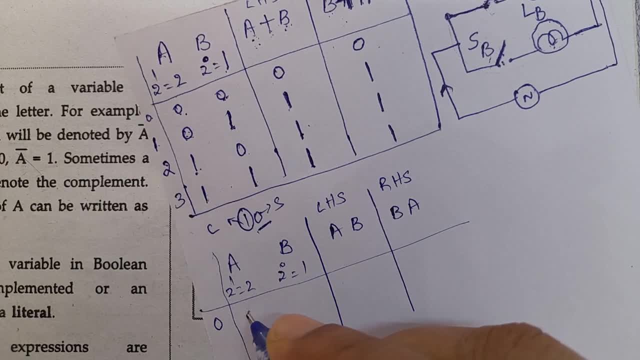 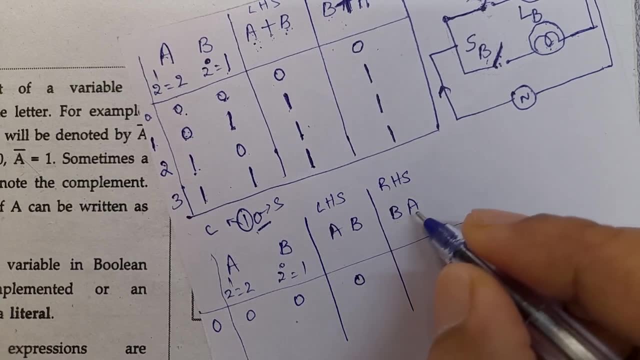 2. power of 1 is 2.. Okay, 0 means both the switches are off. Okay, So A and B. 0 into 0 is 0.. B into A, So B and A is 0 into 0 is 0.. 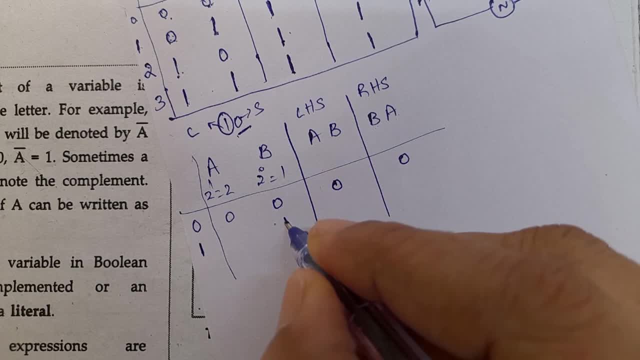 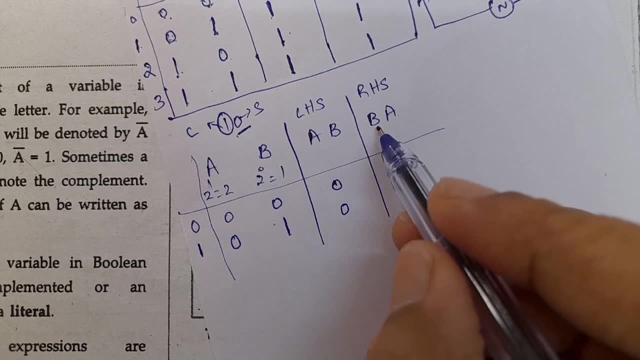 Next 1.. If it is 1, B switch should be on and A switch should be off. A and B: 0 into 1 is 0.. B and A: 1 into 0 is 0.. 2 means 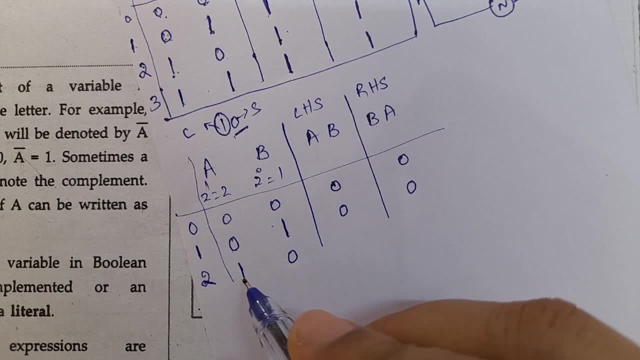 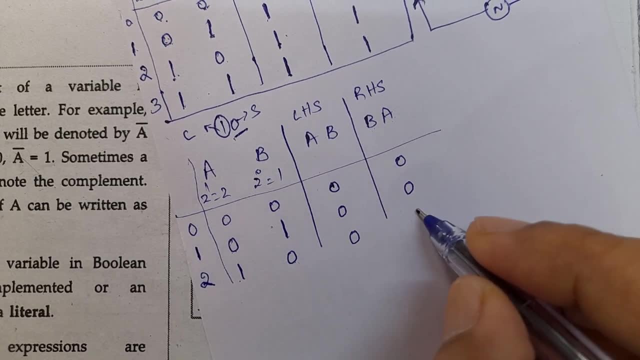 A switch should be on and B switch should be off. A and B: 1 into 0 is 0.. B and A: 0 into 1 is 0. Next, 3.. 3 means 2 plus 1 is 3.. 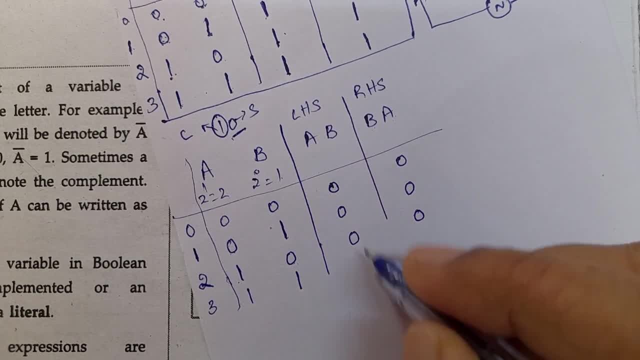 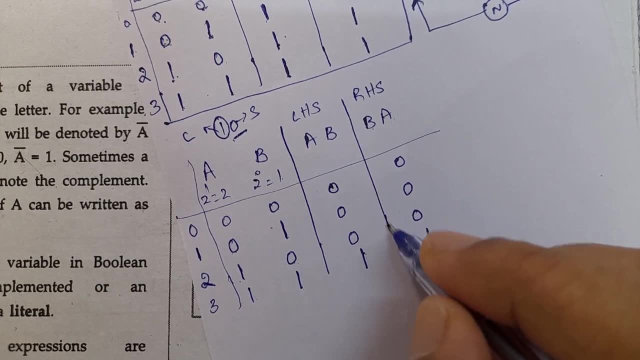 So both the switches should be on. Both are on. So A and B: 1 into 1 is 1.. B and A: 1 into 1 is 1.. So this is for AND operation, AND operation. 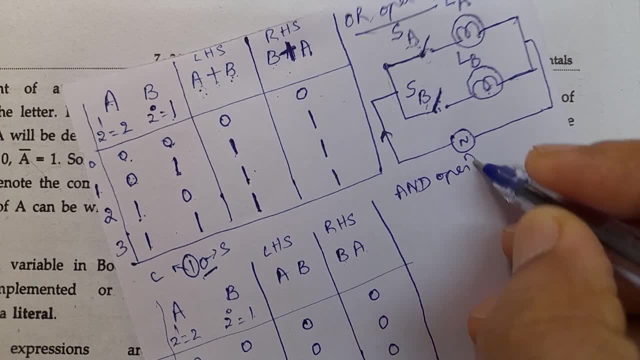 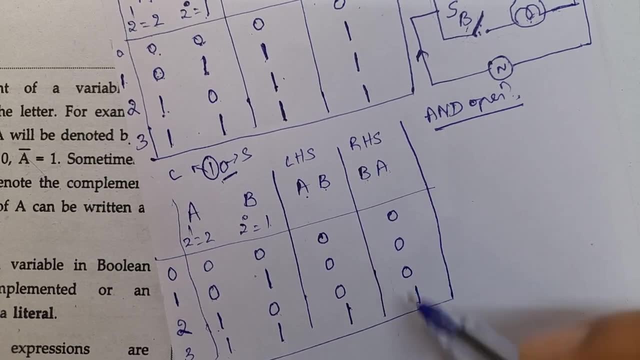 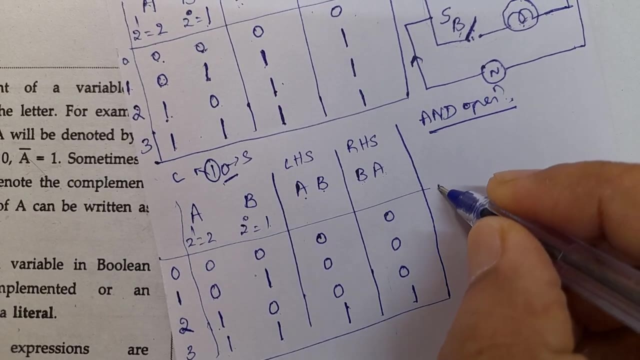 So see here, A and B is same as B and A. Yes, This is for commutative lock. These operations are called series operations. This is A switch, A bulb Switch A And lamp A. So this is A switch. 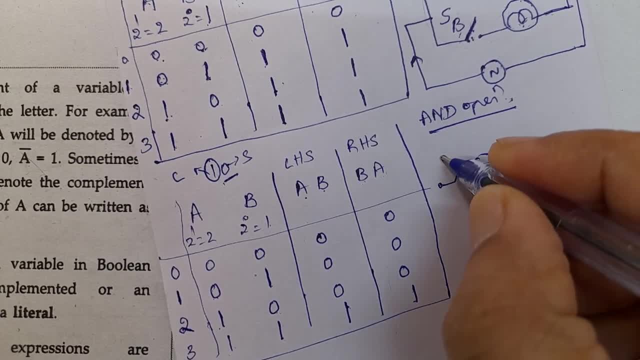 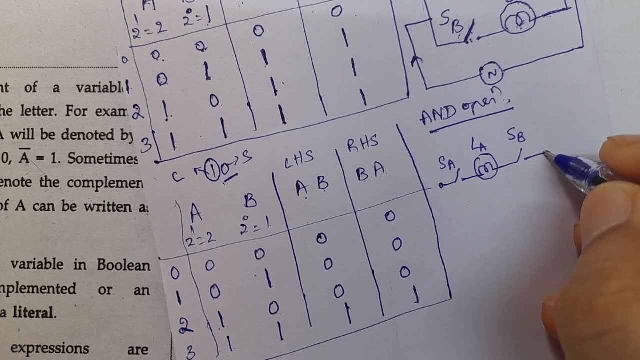 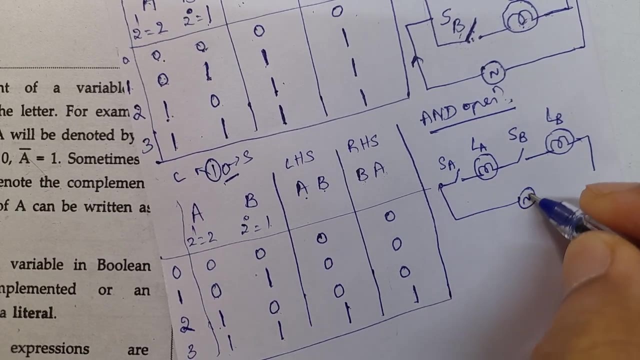 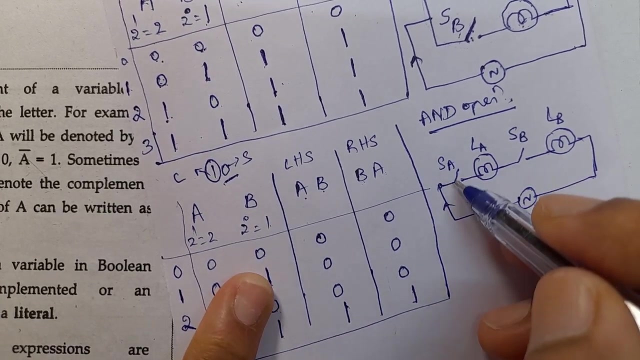 And lamp A. So this is A switch: switch A and lamp A, switch B, lamp B. So AC supply, AC current is flowing. Switch A and switch B. both are open, not closed, So lamps don't glow. 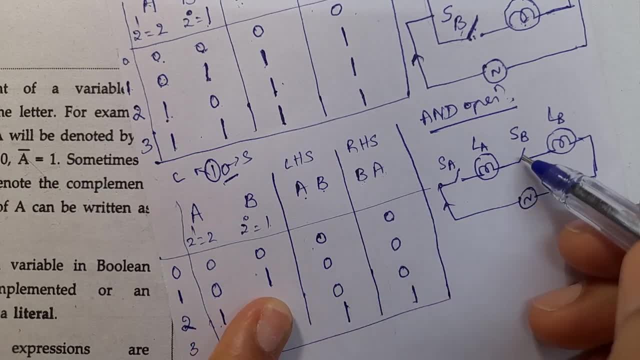 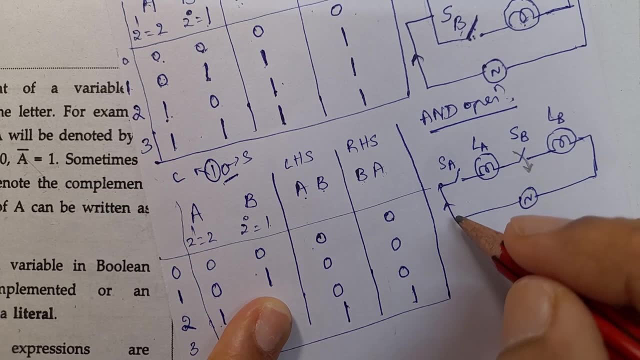 So B switch closed Now. B switch is closed. A switch is open Now. current will come If it is open. no current flows here Now current flows here. even if you close the switch, no current comes Because it is open. 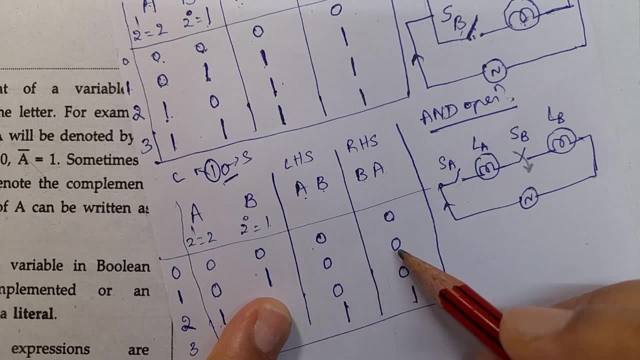 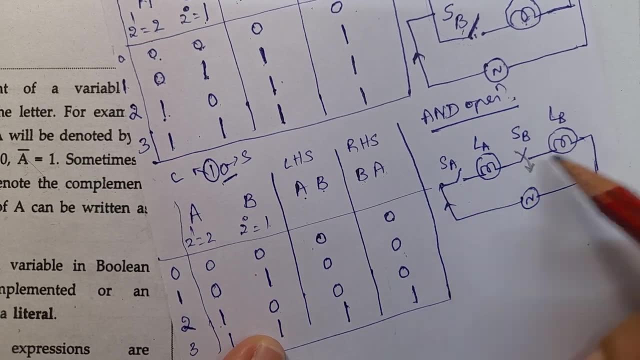 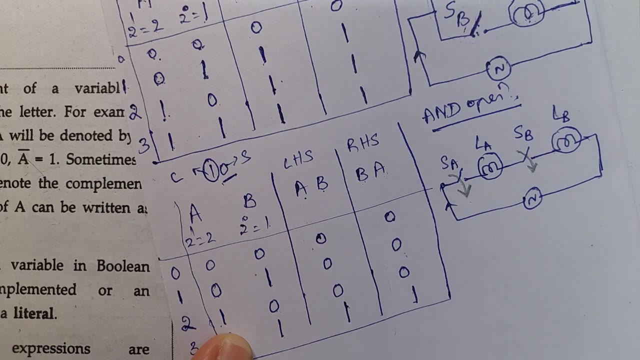 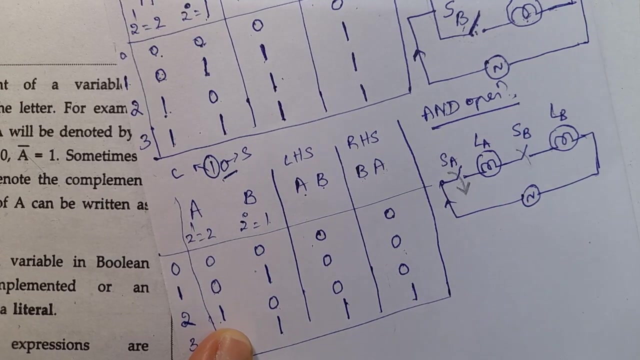 So therefore A and B or B and A is off. So room closed. nimki darkness, either series of connection matter, but a bulb now, okay, either a switch, Oh closer, either be switches in a give it, be switches, so open, I get it. so he's a beast which in my didn't he open, my didn't that I tell. 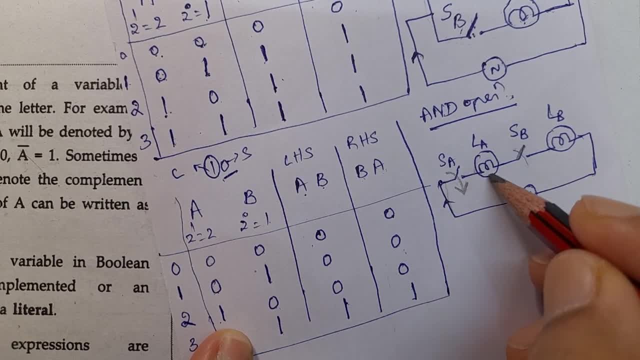 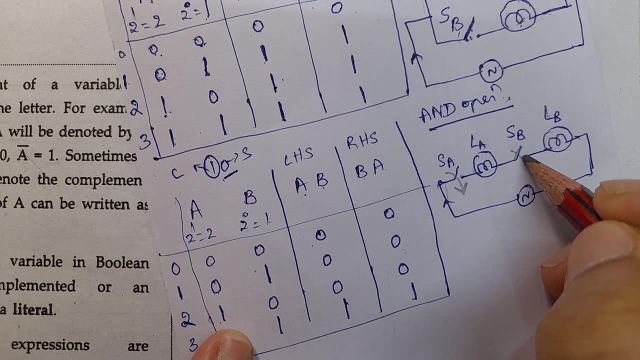 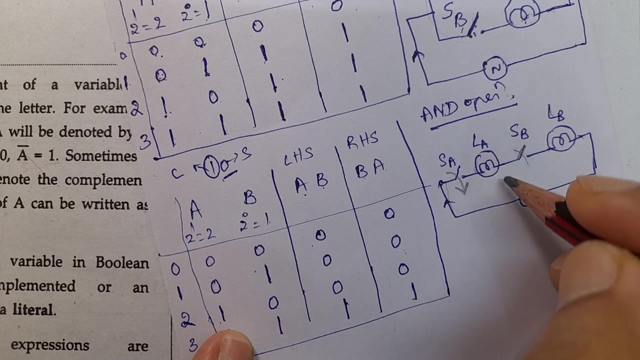 him. so you like current flow. I got that lamp a in a. got there so early blow agouti, love, because he opens. get the other the data la. so you leave current in a. geth a little current. il pass a to patrol go pan若 beg a lava teaches are. 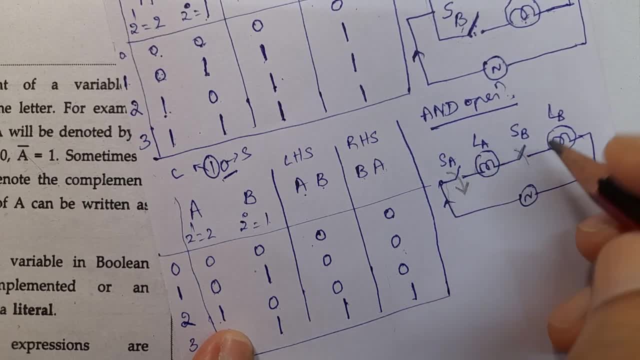 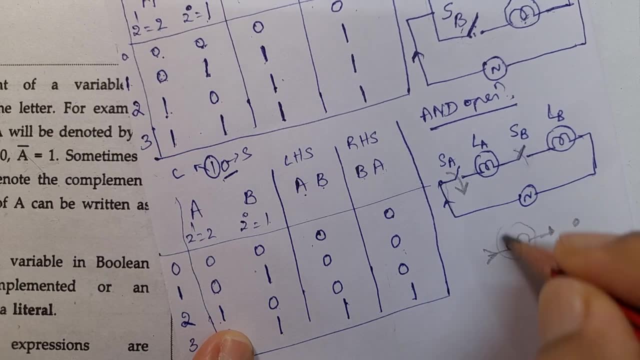 open are pretty. the other in a lamp, a glow out become long time at a lamp though. one end al current pass, other way another end: all you open a pagar odrin the lamp in a geth, a glow. agouti de la la open agar oder in the open circle, only there. 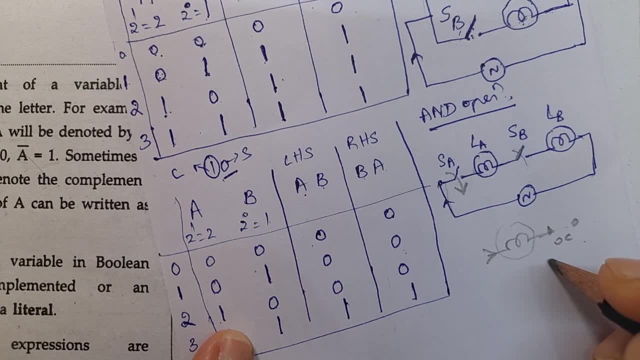 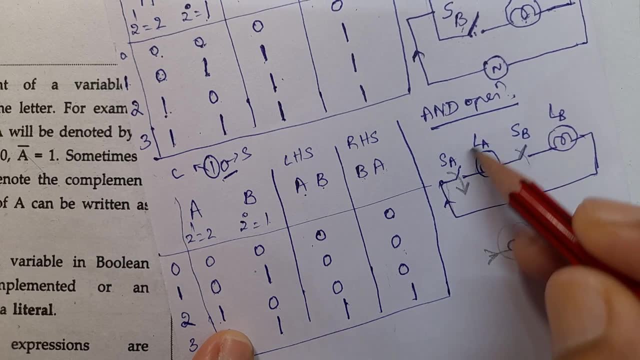 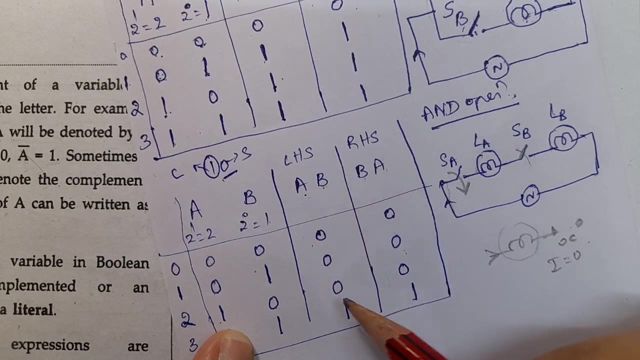 is no current flows, the data law current on the circuit and the here we go, current flows, here we go, current flows, here we go. What is the current Minimum current? So here the lamp does not glow, So here also the lamp does not glow. Here it is open, So the lamp does not glow. So A and B and B and A, both are off. 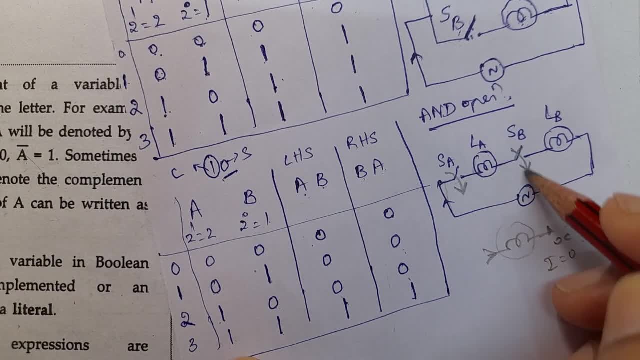 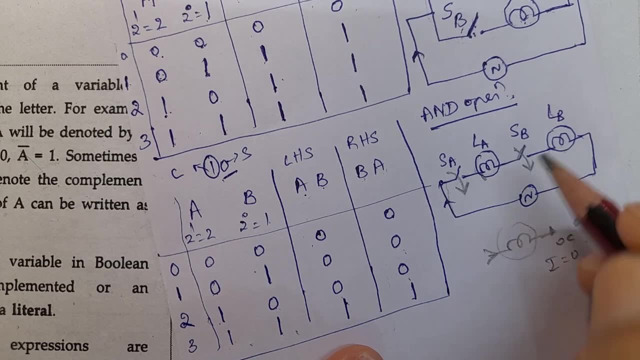 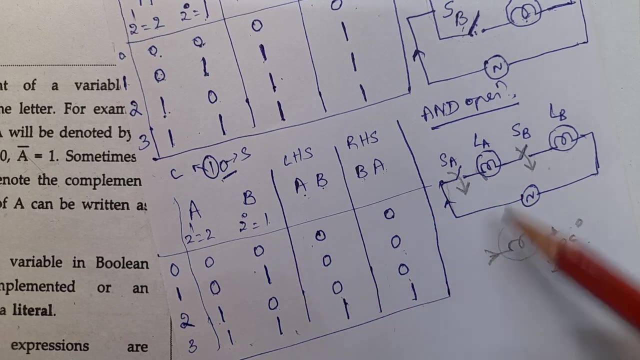 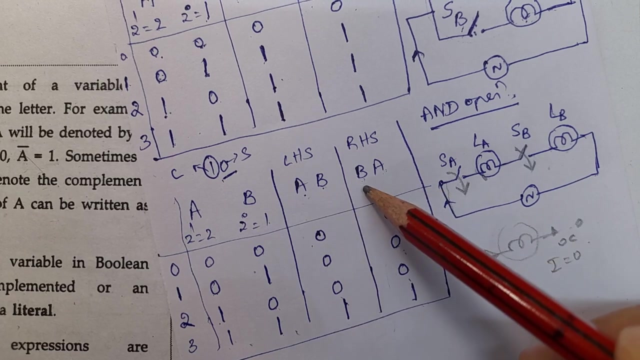 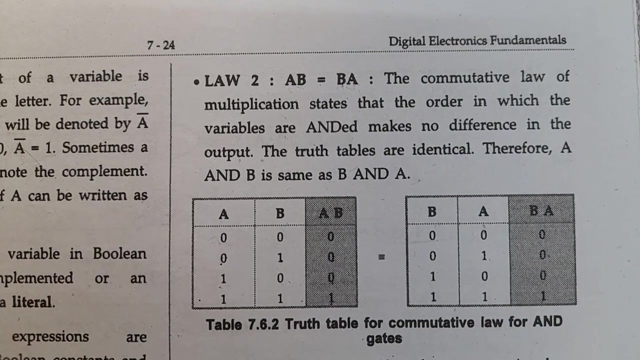 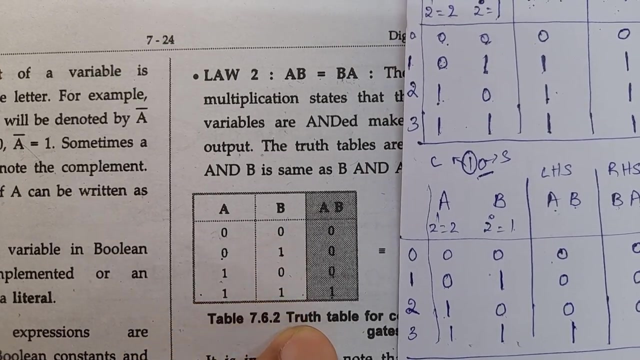 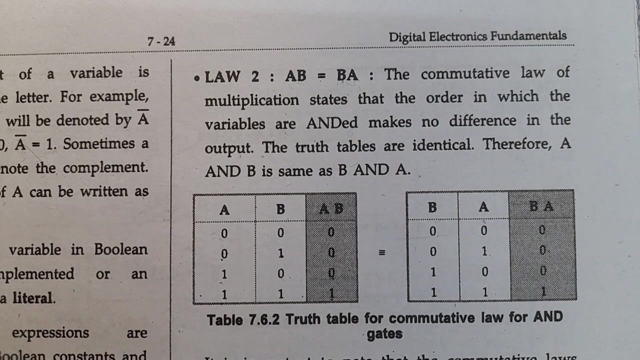 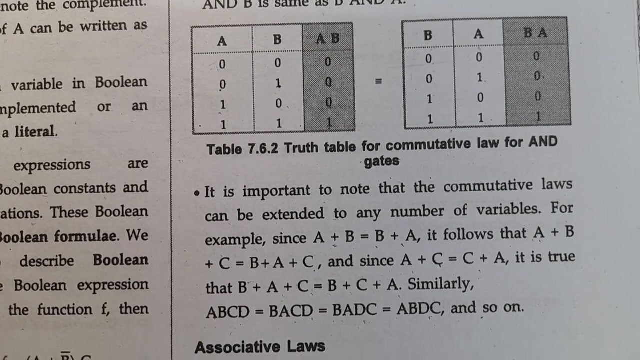 Okay. Next, both the switches are closed. So this is the end operation series connection. So A and B is the same as B and A. Okay, See the table. Table Table note back. So A and B is 0001 and B and A is 0001.. Okay To table 7.6.2. to table for commutative law for: AND gates. Next. 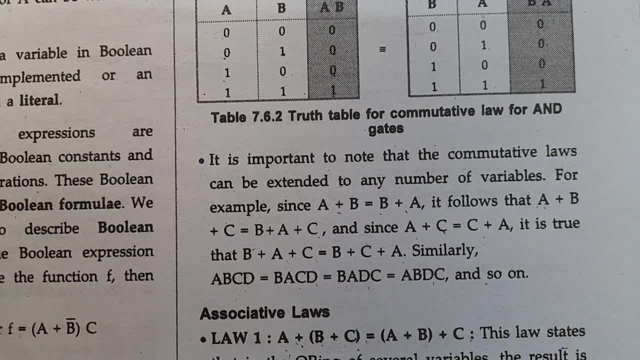 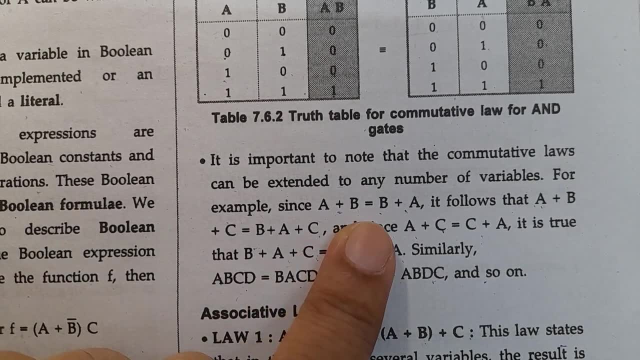 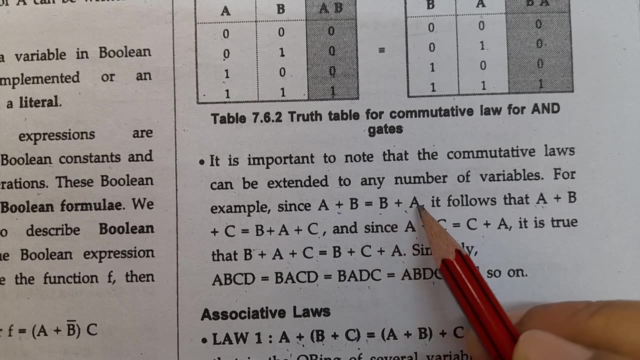 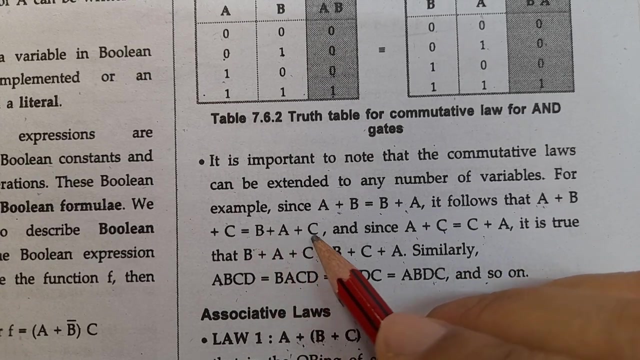 It is important to note that the commutative laws can be extended to any number of variables. For example, since A plus B is A or B and A or B is the same as B or A, It follows that A or B or C is the same as B or A or C. And since A or C is the same as C or A, 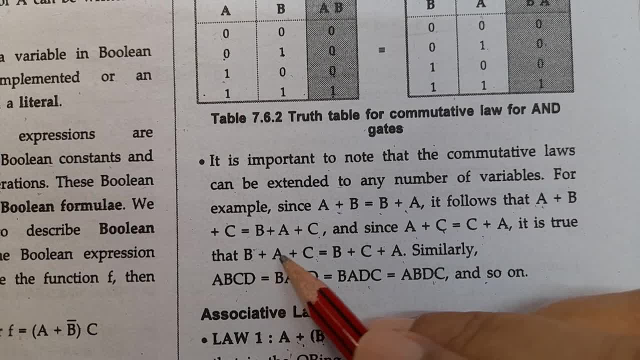 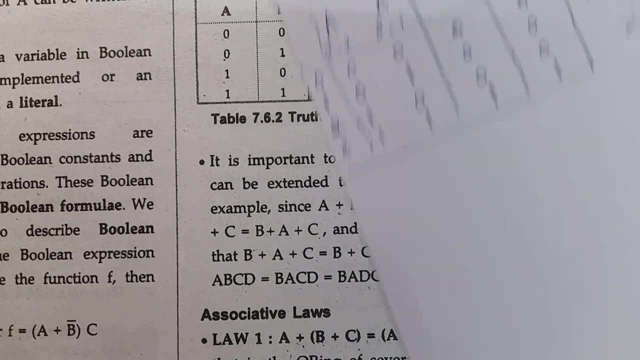 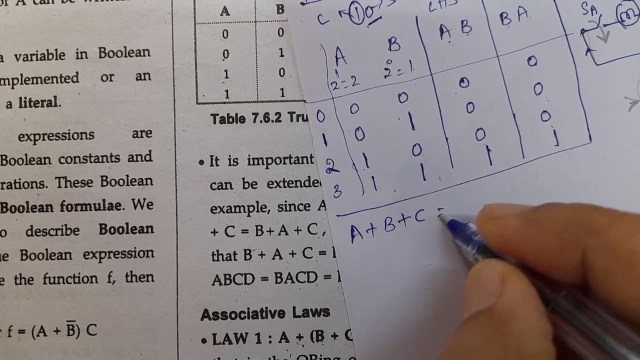 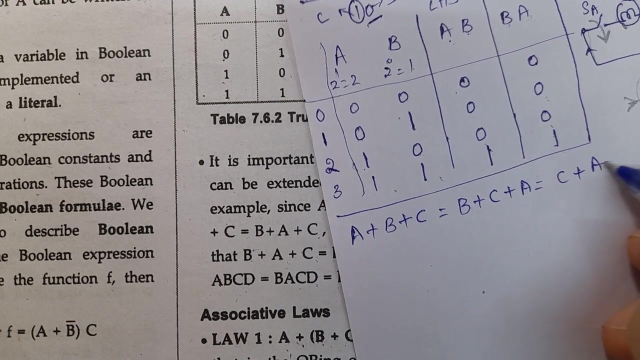 Okay, B or C or A, And then Now we have seen only two variables. Suppose three variables: A or B or C, Equal to B or C, or A Or C or A or B. All are same, All are same. 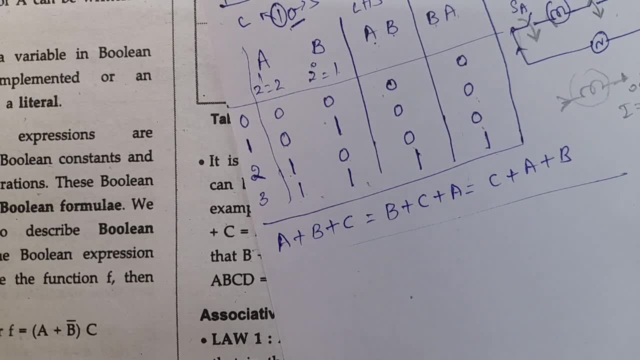 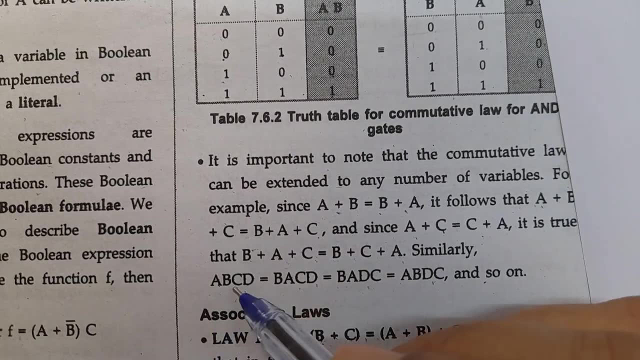 These are all same R operations. Commit to law for R operations Next to A, B, C, D, A and B and C and D Is same as B and A and C and D Is same as B and A and D and C. 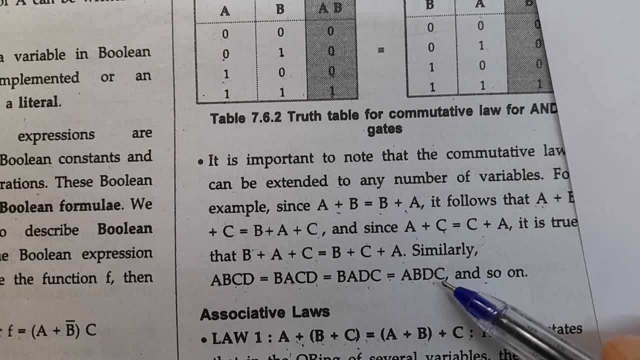 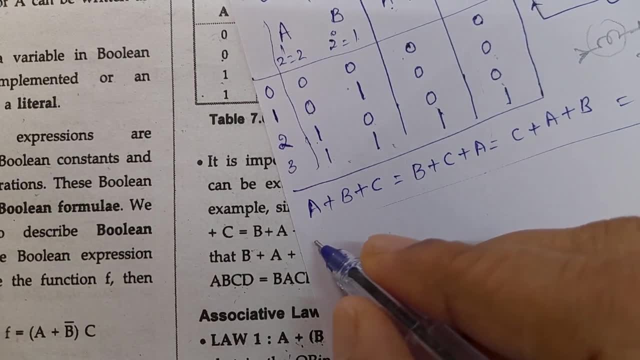 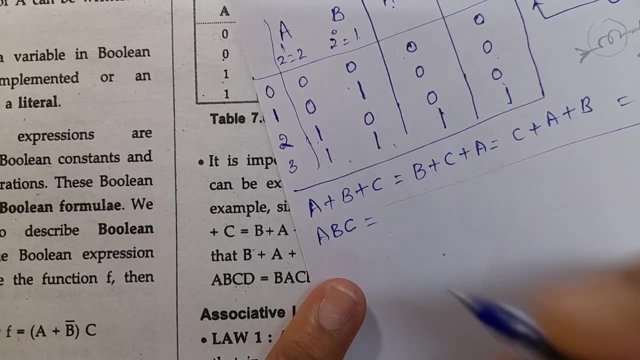 Is same as A and B and D and C And so on. This is for R operation. Ok, Next to AND operation, A and B and C. I will take three variables: First, Next to B, and C and A. 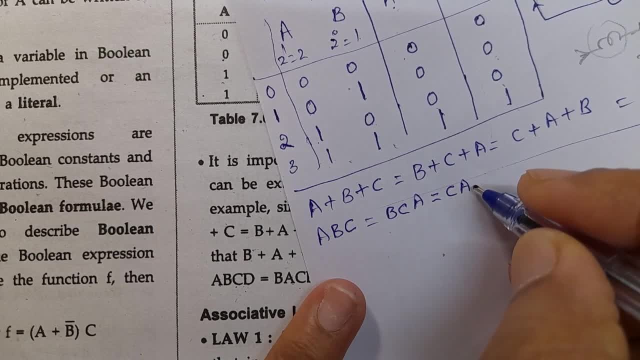 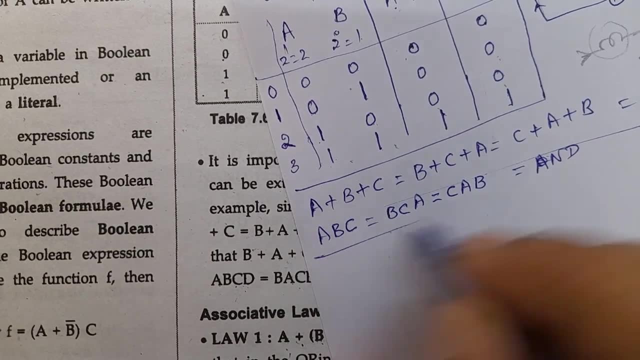 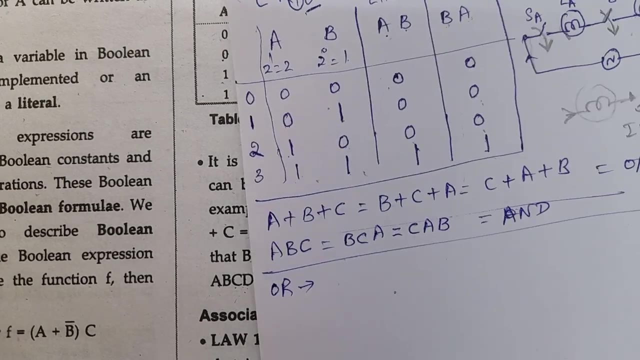 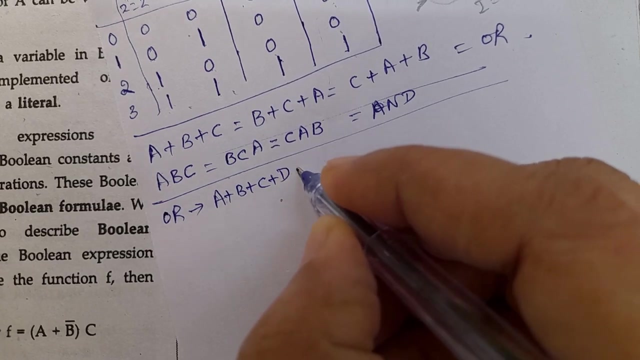 Next is same as C and A and B. So these are the AND operation. So next to Four variables, R operations. For R operation, Four variables Are present, So A or B or C or D Is same as. 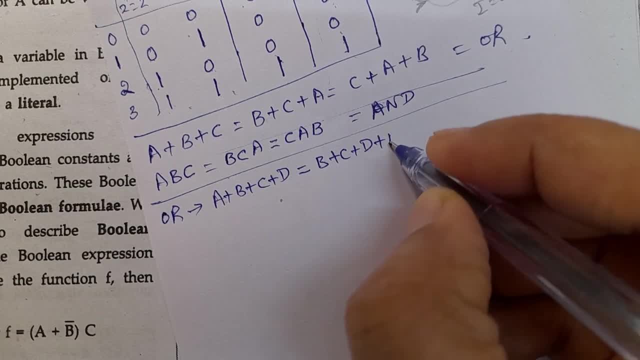 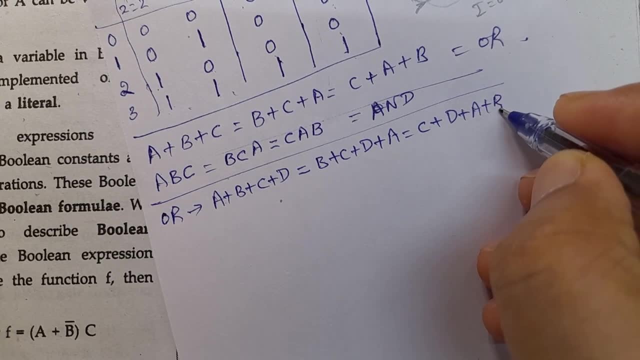 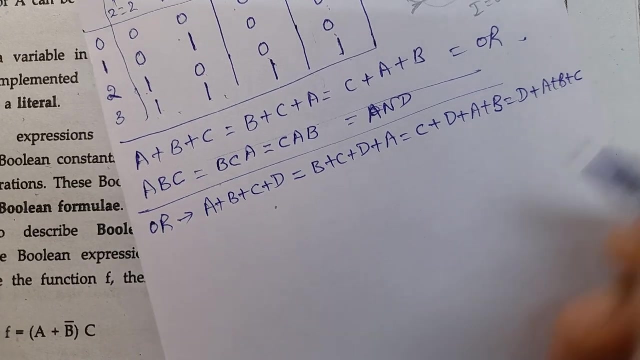 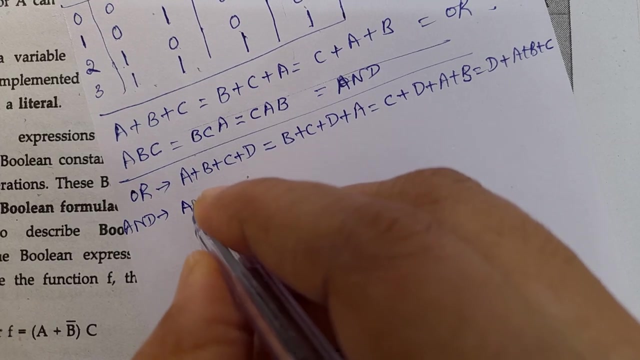 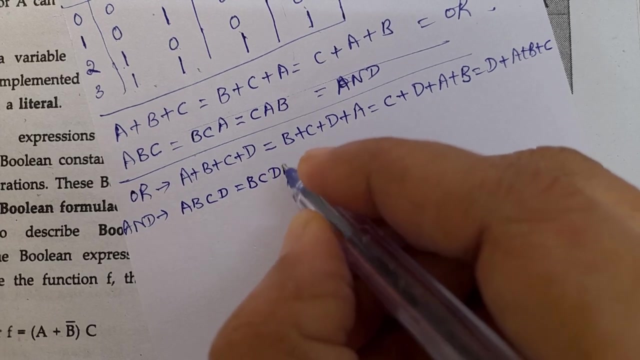 B or C or D or A Is same as C or D or A or B Is same as D or A or B or C. Next to AND operation: A and B and C and D Is same as B and C and D and A. 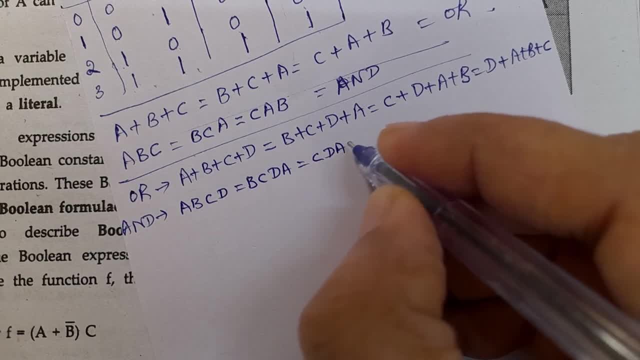 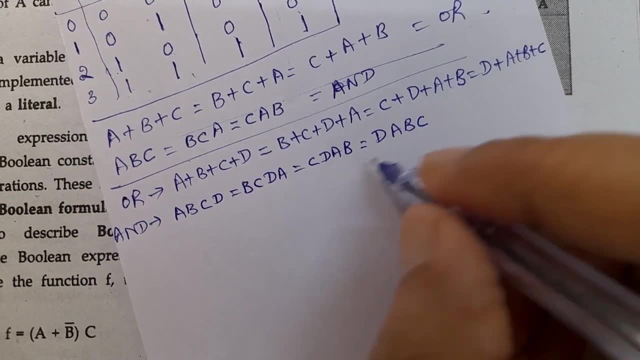 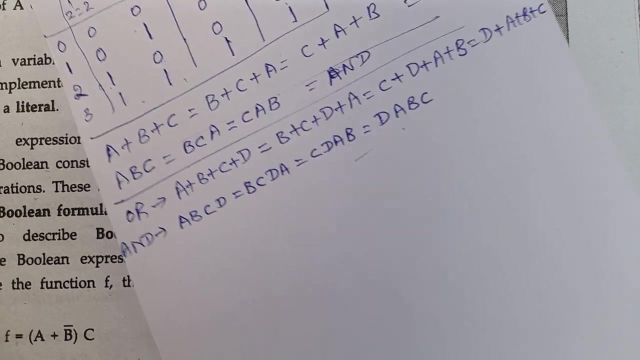 Is same as C and D, and A and B Is same as D and A, and B and C. So these are the AND operation. This is for R operation. How many variables? So that is same. Next, Associative law. 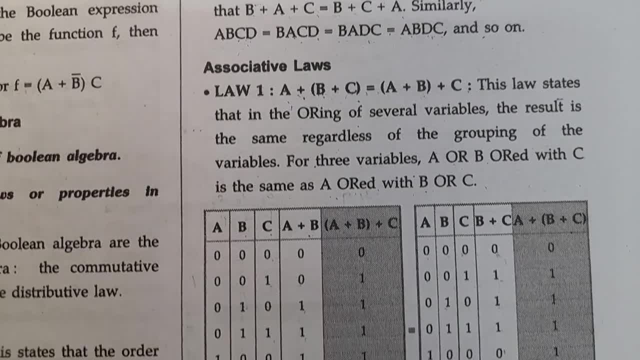 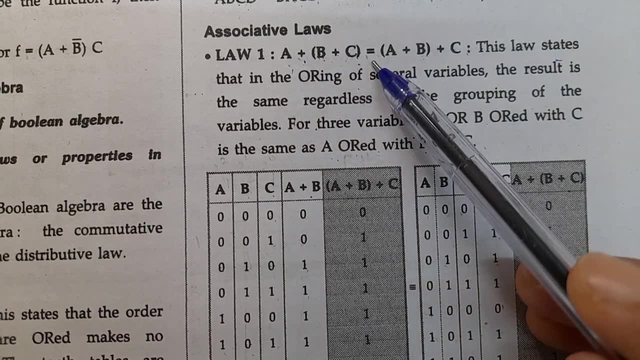 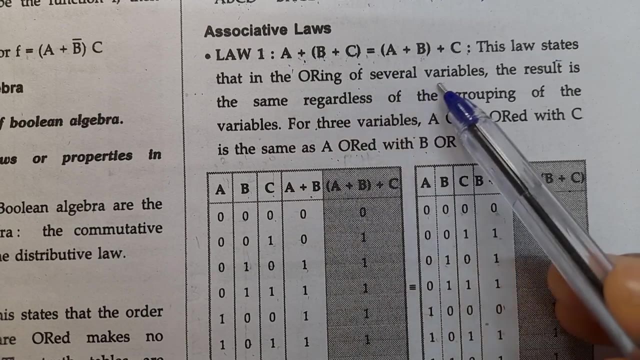 Second law Is associated with Associative law, Law 1. So A or B or C Is same as A or B or C. This law states that In the ORing of several variables The result is the same. 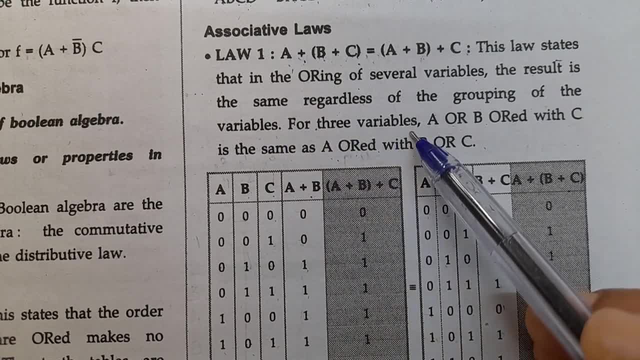 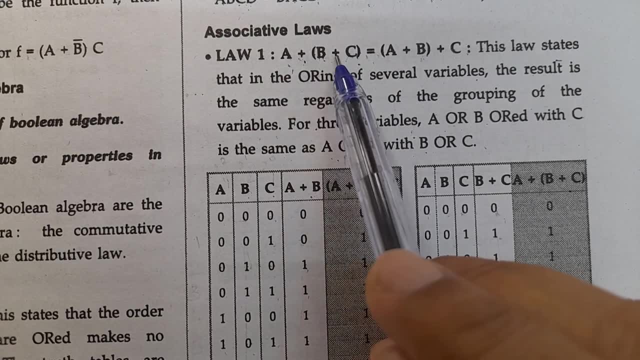 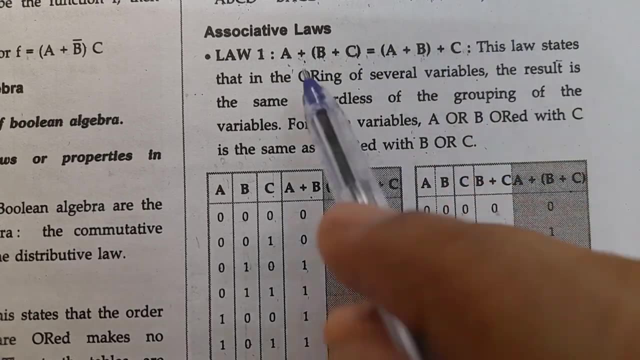 Regardless of the grouping of the variables For three variables: A or B, A or B or C, B or C. A or B or C Is the same as A ORed with B With C. That means first what we have to do. 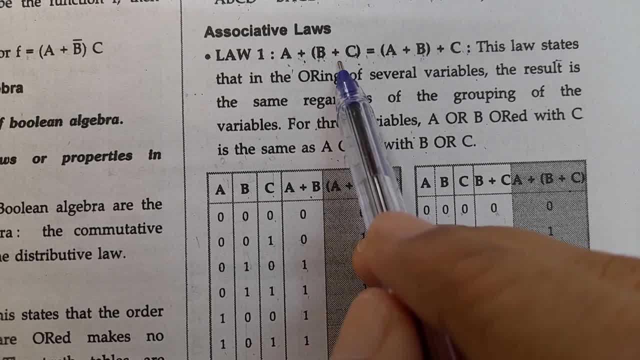 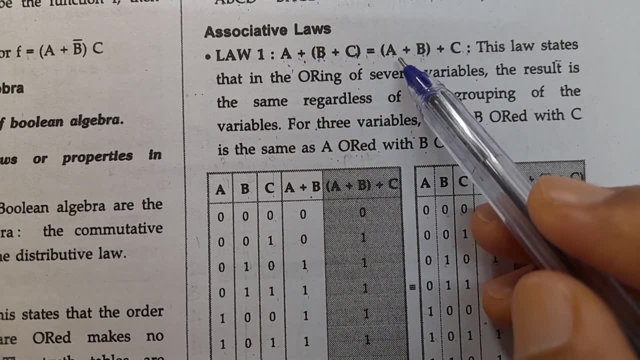 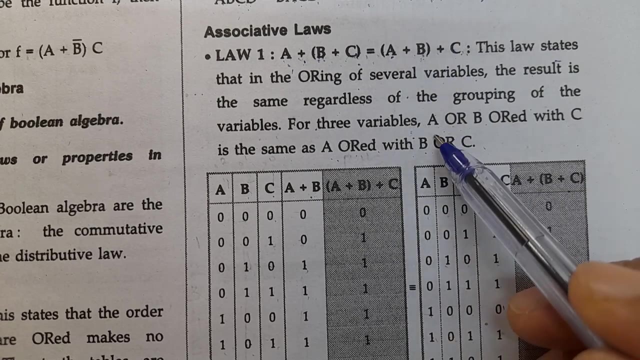 B and C Have to be ORed. What will be the result? That has to be ORed with A. This is the first step. Where A is And where B is, First OR operation has to be done. That means C has to be ORed with C. 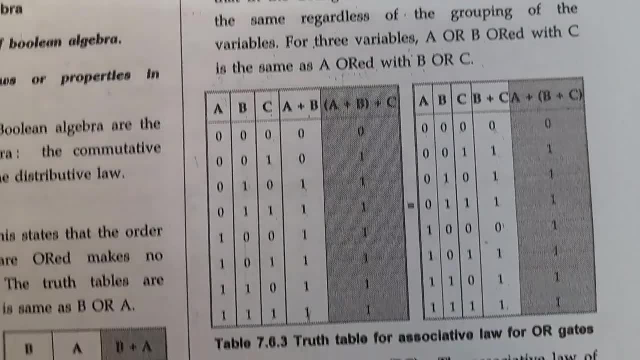 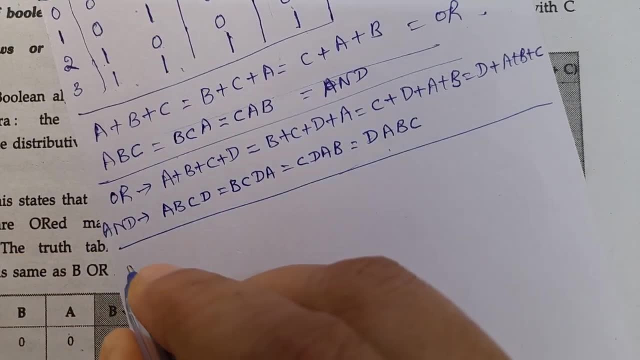 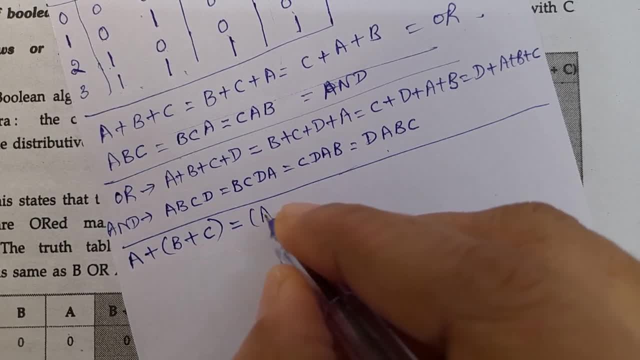 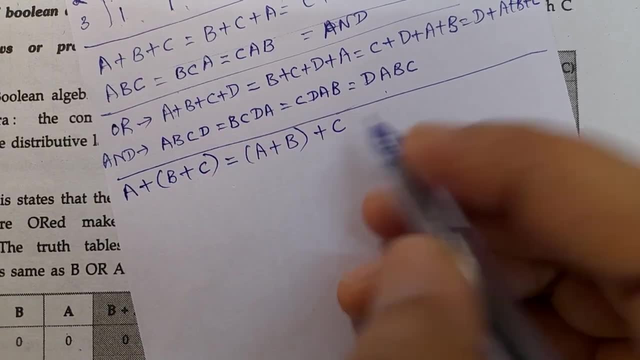 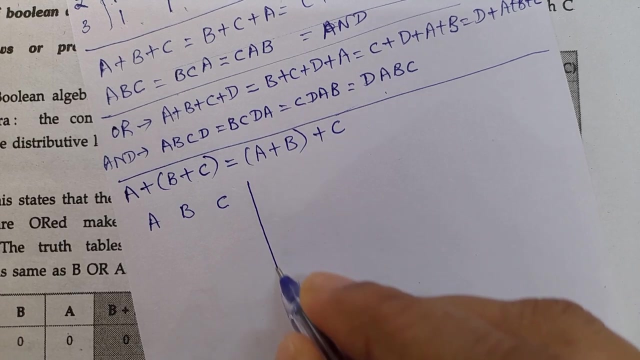 Is the same as A, ORed with B OR C Is the same as This is LHS, This is the RHS. So this is first. A, B, C are three variables. Next, first thing we have to do is B plus C, That is, B OR with C. 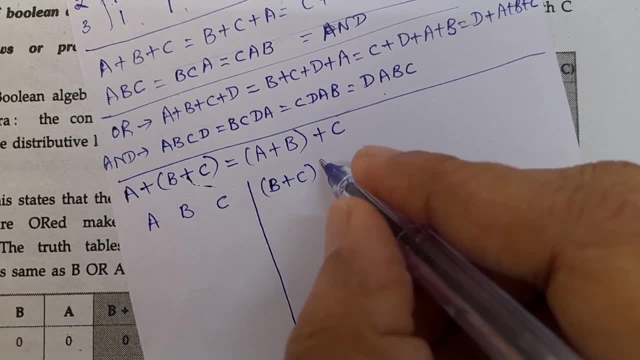 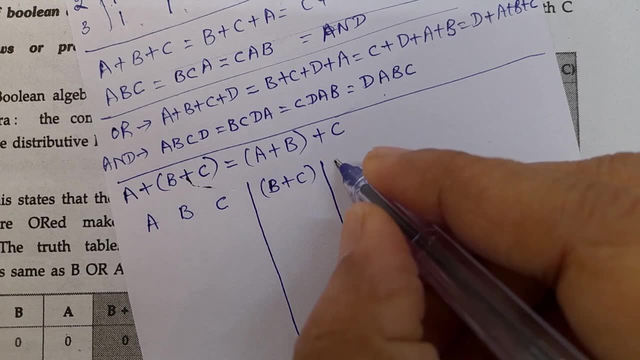 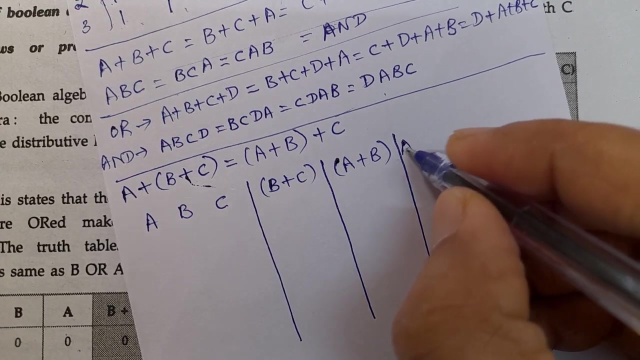 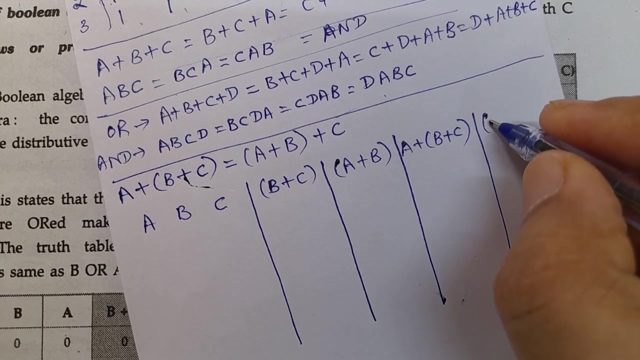 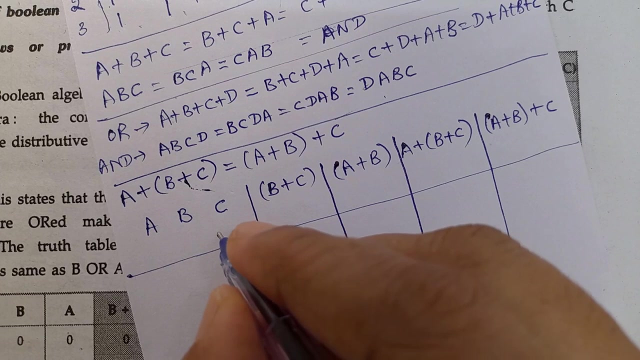 B OR with C. So now let's do LHS A OR with B, A OR with B. Let's do this Next in: LHS A OR B OR with C is the same as A OR with B or C. So 2 power of 0 is 1.. 2 power of 1 is 2.. 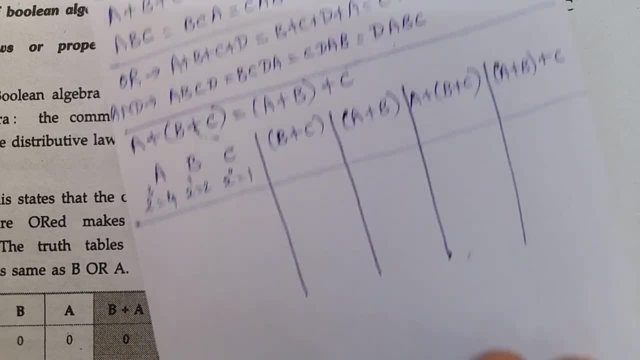 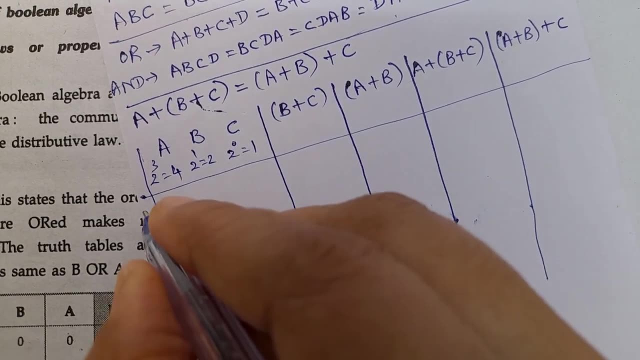 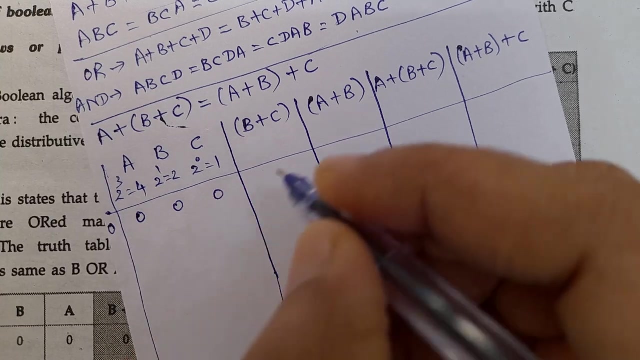 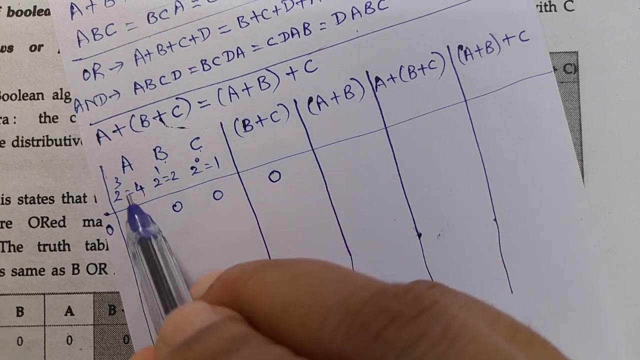 2, power of 3 is 4.. So next, 0.. 0 means all the inputs are 0.. 0, 0, 0.. So B OR with C, OR operation is 0.. A OR with B, So that is also 0.. 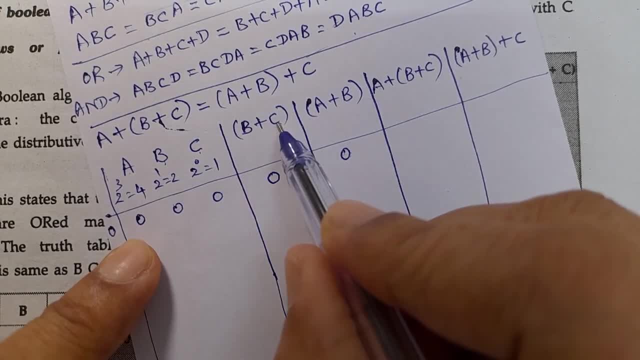 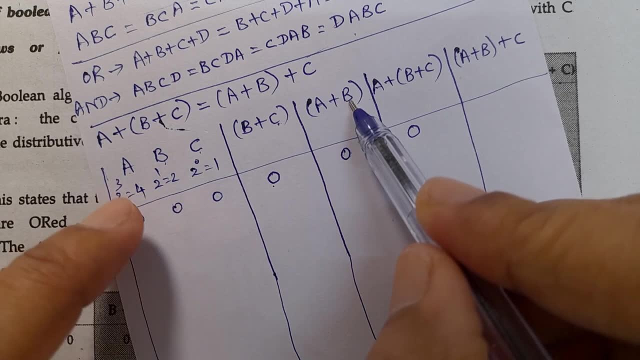 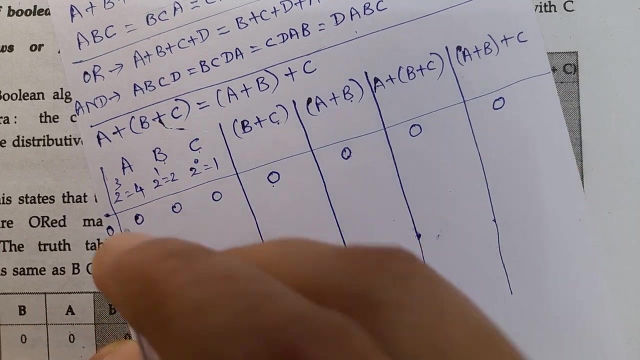 Next B OR with C. So OR operation is 0.. Next A OR with B. A OR with B. ORD with B is 0.. Along with that, C is ORD. operation is 0.. Next 1.. 1 means this C should be ON. 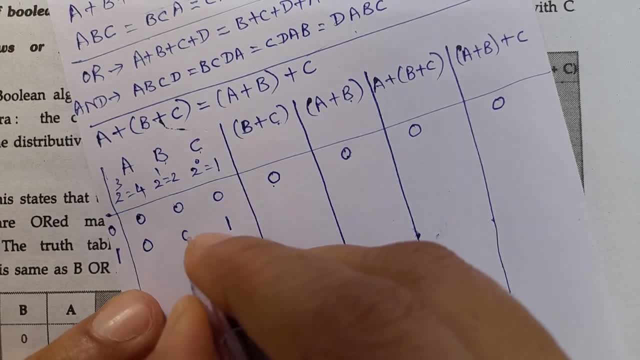 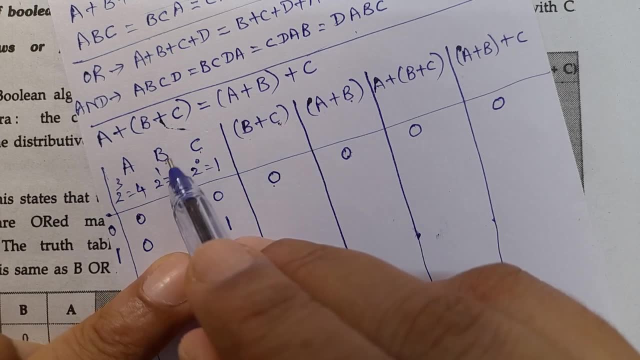 Here: 1 is not there, C is ON, Rest two should be OFF. Two inputs remaining. two inputs are 0.. So B ORD C. B ORD C means 0 plus 1 is 1.. Next A ORD with B. 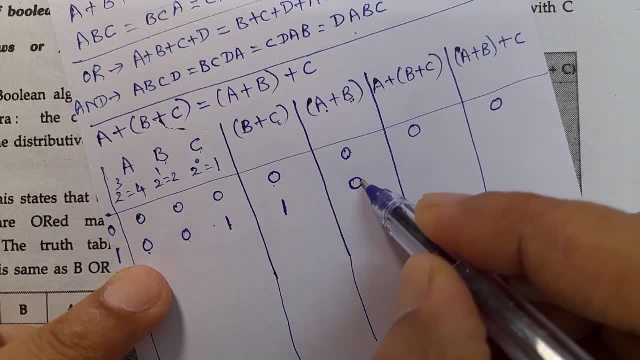 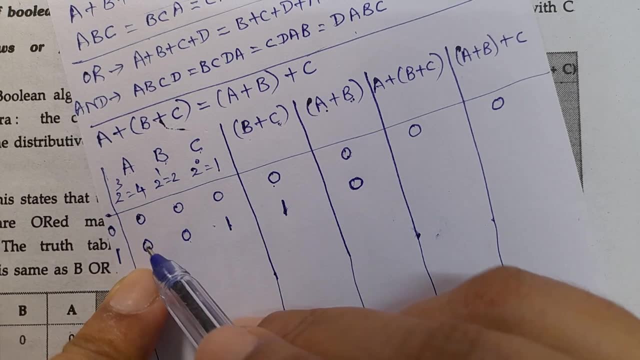 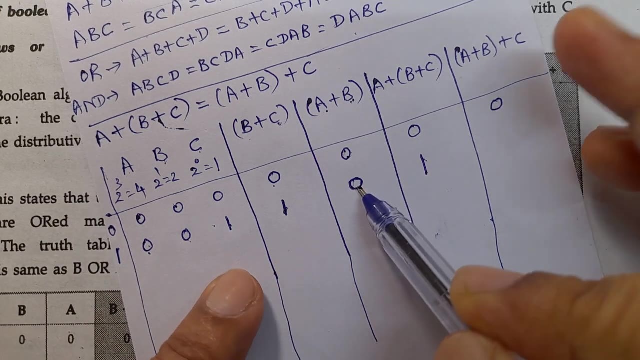 A ORD with B: 0 plus 0 is 0.. Next B ORD with C is 1.. Next, along with that, A, 0 plus 1 is 1.. Next A plus B is 0.. 0 plus C. 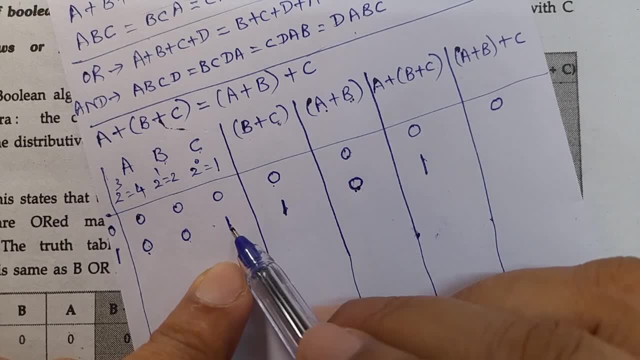 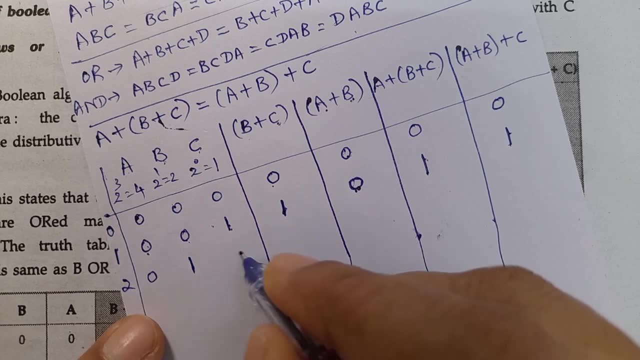 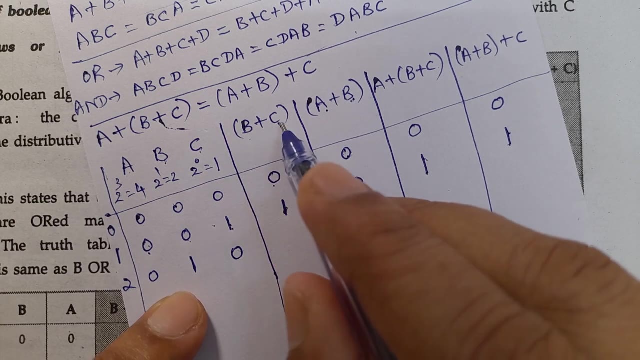 If you say plus C, it is 1.. 0, plus 1 is 1.. Next 2. 2 means this should be ON Input A and input C should be OFF. Next B plus C. B ORD B ORD C. 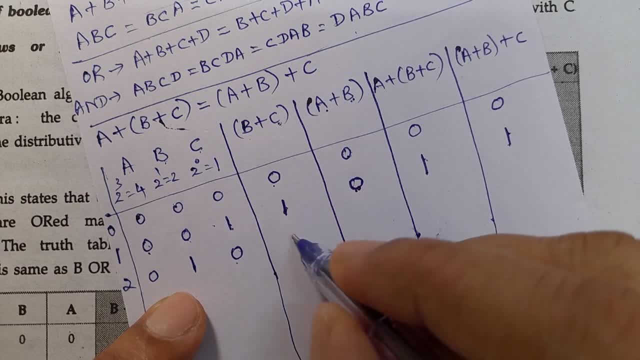 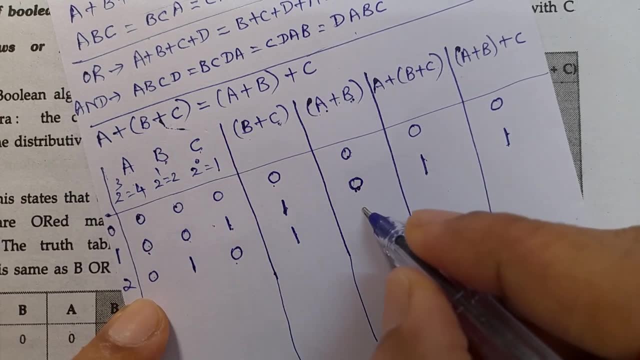 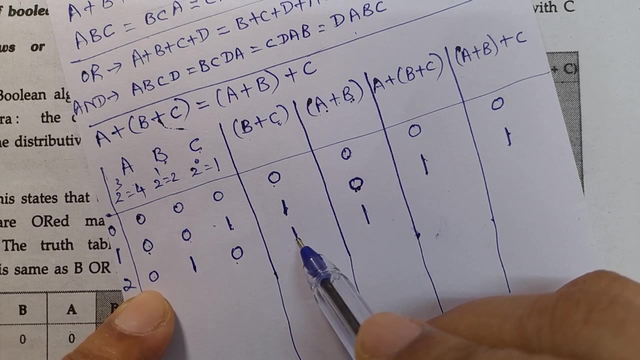 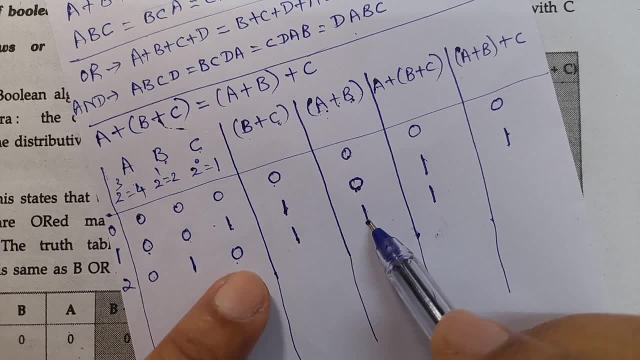 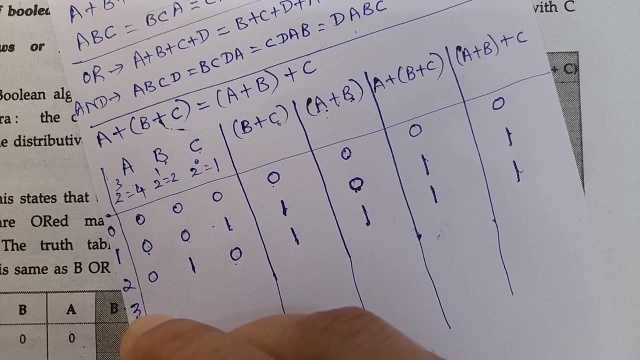 A ORD with B is 1. And C is 0.. 1 plus 0 is 1.. 1 plus 0 is 1.. Next 3. 3 means 2 plus 1.. B and C must be on. 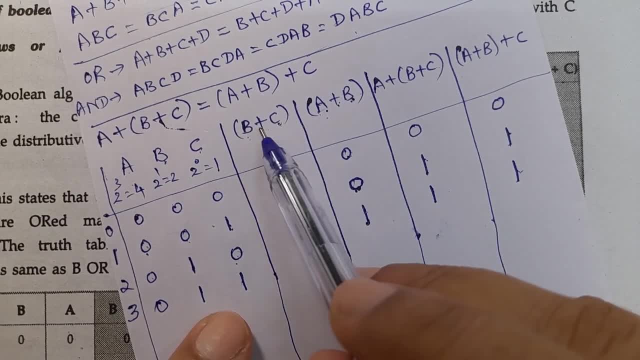 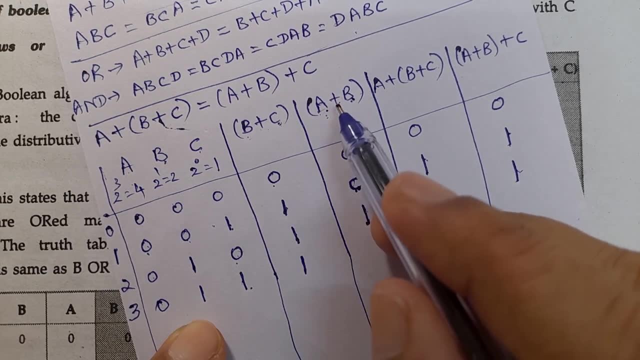 A must be off. B ORD with C: 1 plus 1 is 2.. 1 must be on. A ORD with B. A ORD with B: 0 plus 1 is 1.. A ORD with B. A ORD with B. 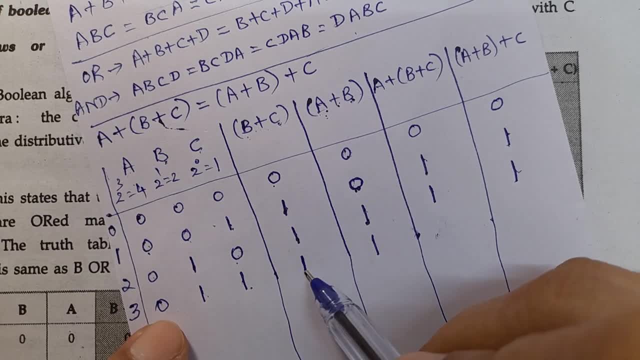 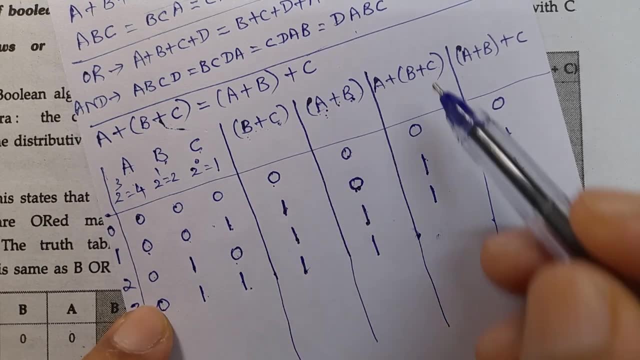 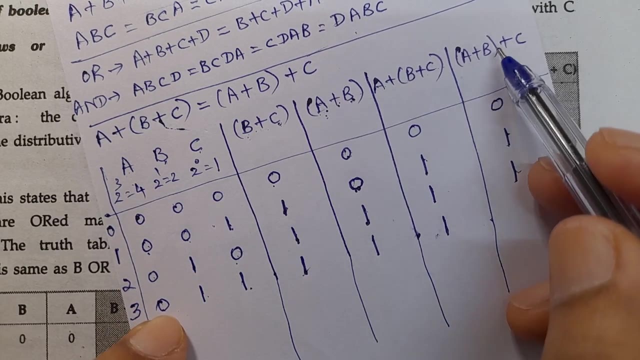 0 plus 1 is 1.. b or with c is 1 or c a- sorry- or a b. first a is 0, b or with c is 1, so 0 plus 1 is 1, next a or with b is 1 or c 1. 1 plus 1 is 2. 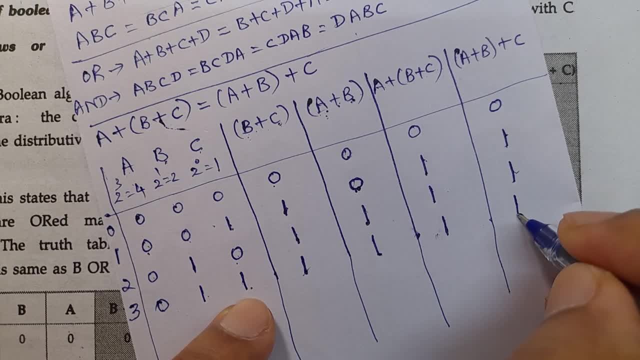 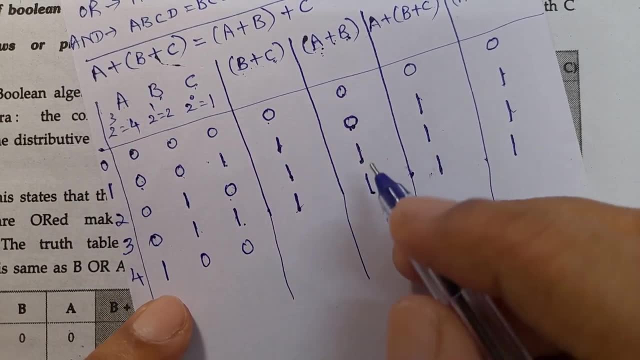 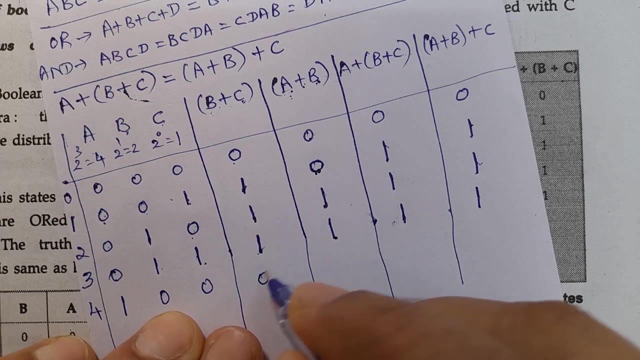 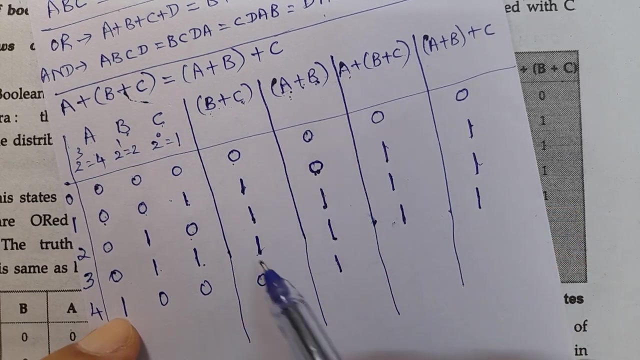 that means if both are on, then output is on. next 4. a is on, b is off, so b. or with c. b or with c is 0 plus 0 is 0. a or with b is 1 or c is 1. a or with b is 0, so 1 or c is 1. 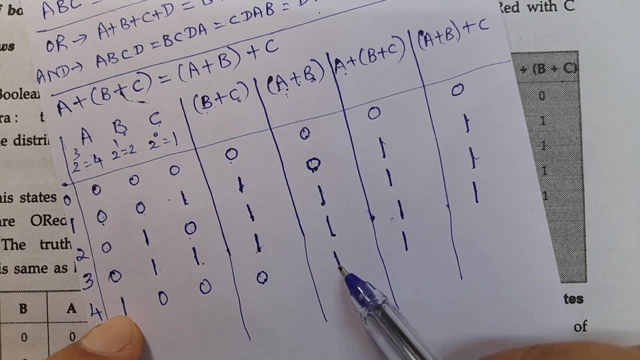 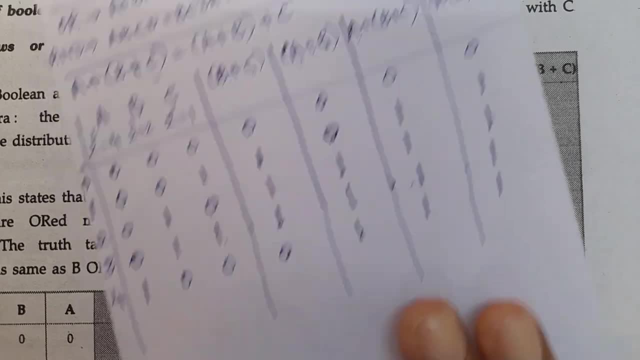 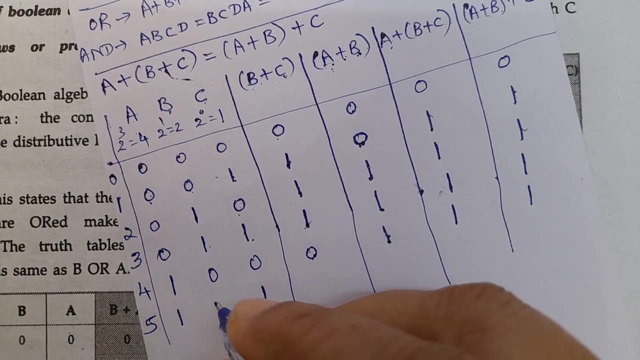 now Next: a odd with b. a odd with b is 1.. Or c: 1 plus 0 is 1.. Next fifth: 4.. That means a variable c variable should be on, b should be off. 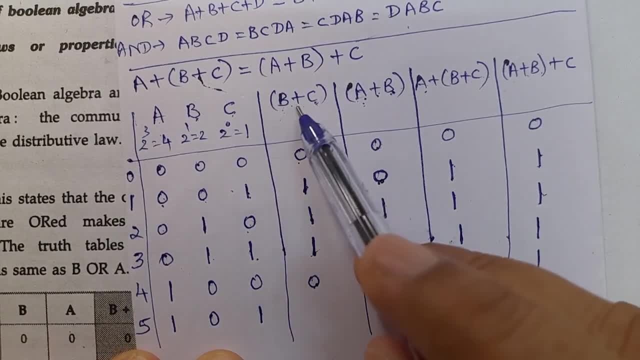 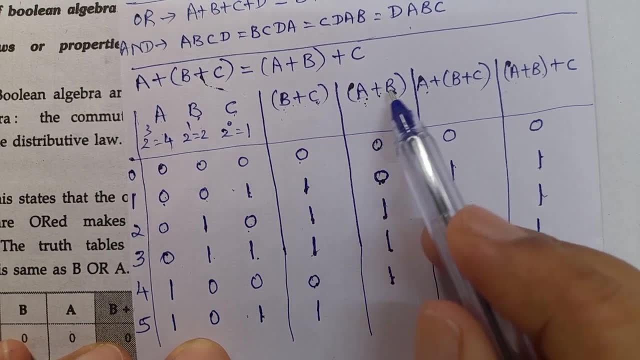 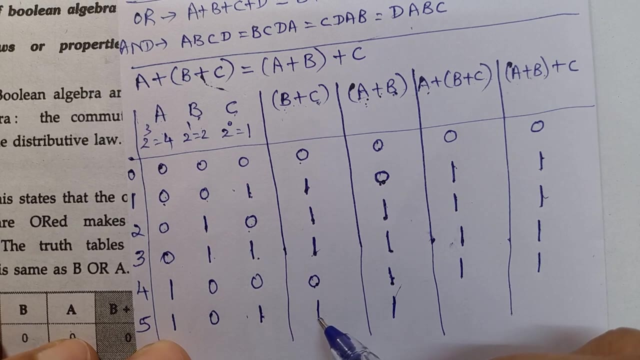 So b plus b odd with c, b odd with c. So 0 plus 1 is 1.. Next a odd with b: 1 plus 0 is 1.. Next a b odd with c, 1 plus 1 is: 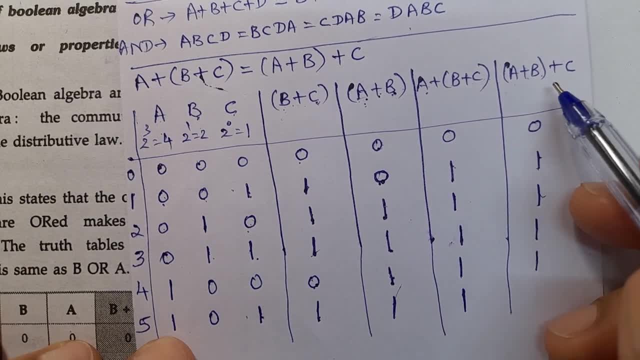 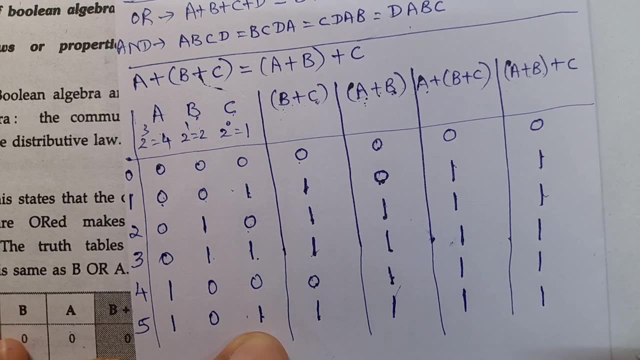 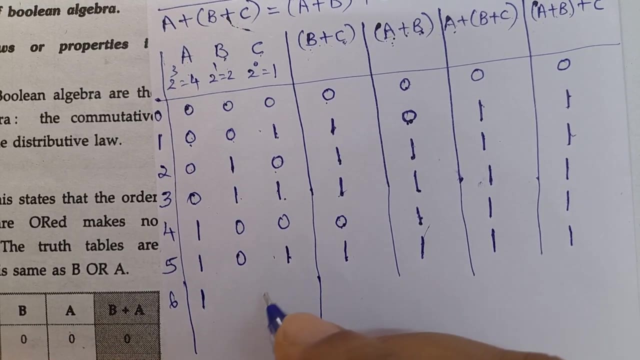 That means both are on. That means this is on. a. odd with b is 1.. c is 1.. Both are on, So this is output Next sixth, So 6 means 4.. a should be on, b should be on, So c should be off. 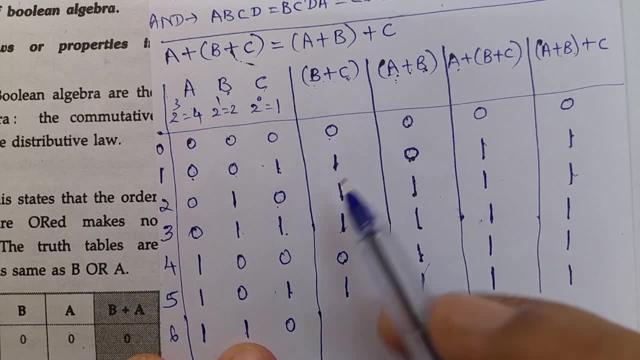 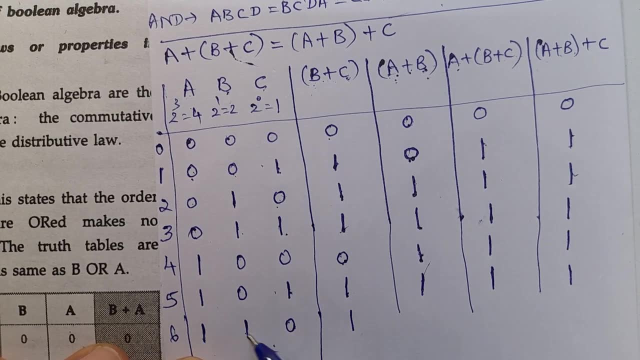 b odd with c: 1 plus 0 is 1.. a odd with b: 1 plus. both are on, So this is on. a. b odd with c: Both are on. This is on. This is on, So this is on. 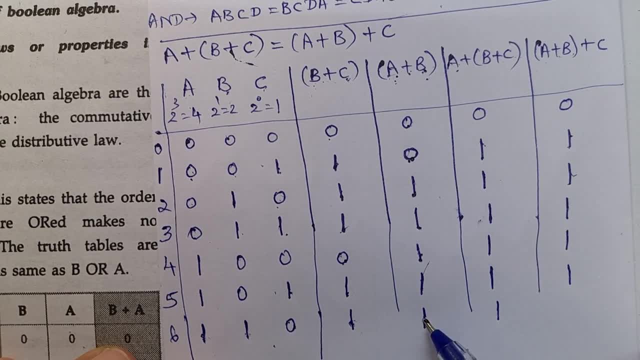 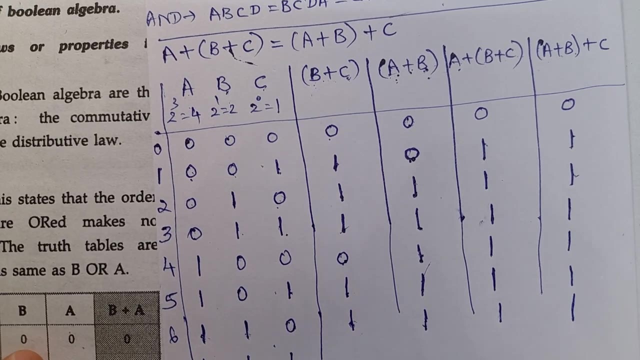 a odd with b is on, c is off, No problem. so 1 plus 0 is 1.. Next 7 means 4.. 4 plus 2 is 6.. 6 plus 1 is 7.. 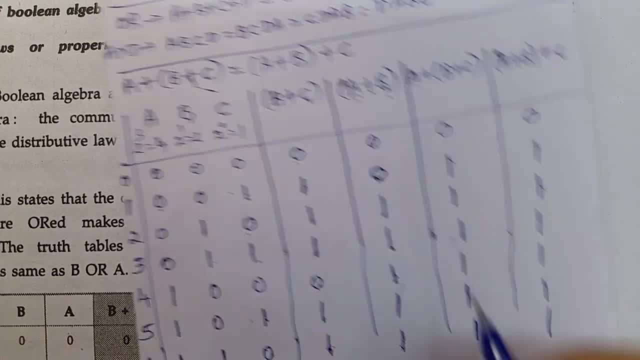 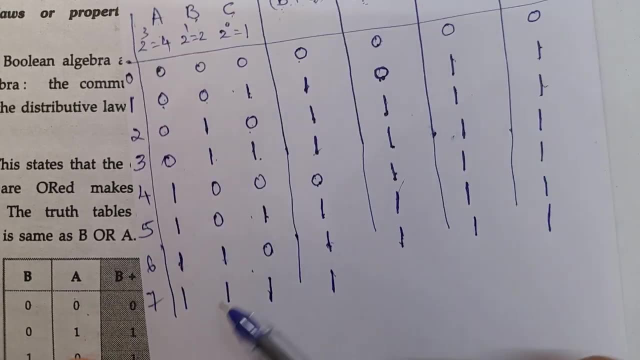 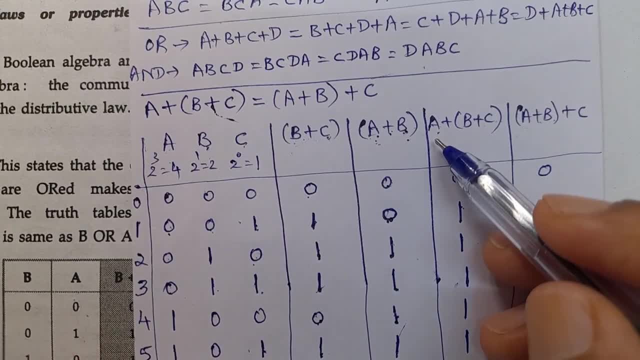 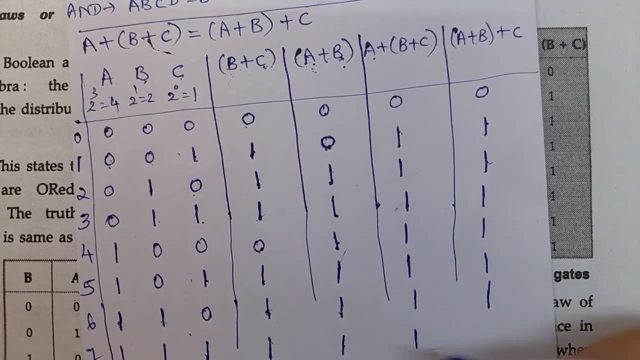 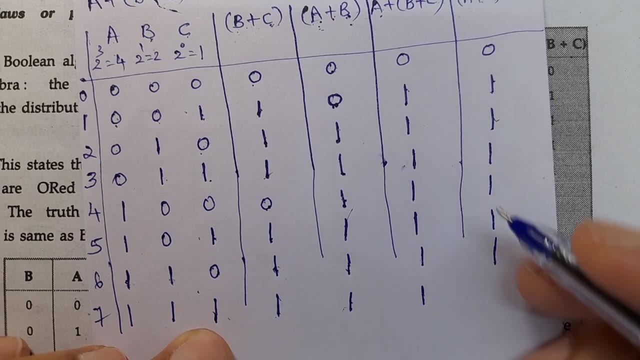 A odd with b, A odd with b, A odd with b on. so either put on another, so a on again B or with the C is on. both are on. illa coulda another day, a or with B, so that is on. C is also on, both are on. so 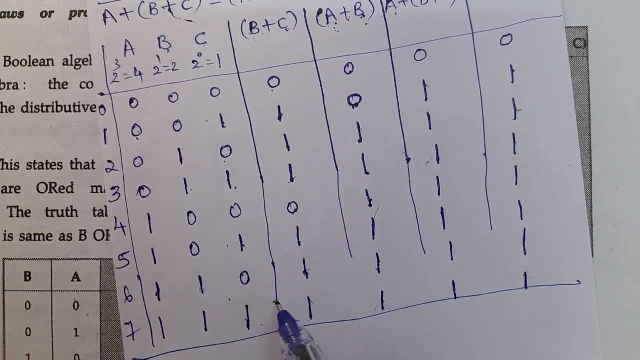 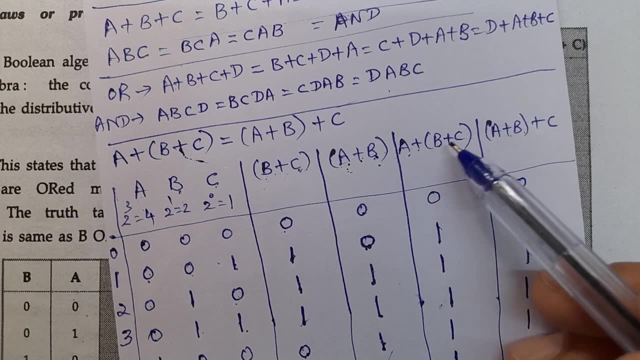 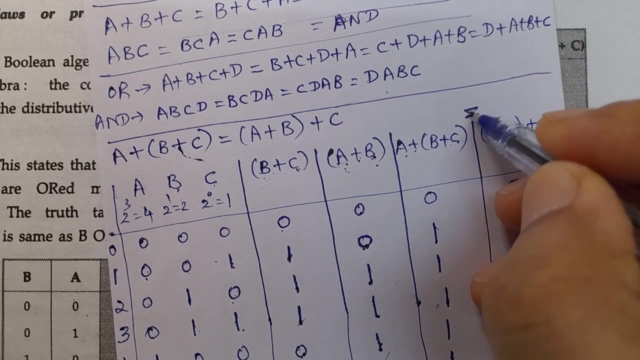 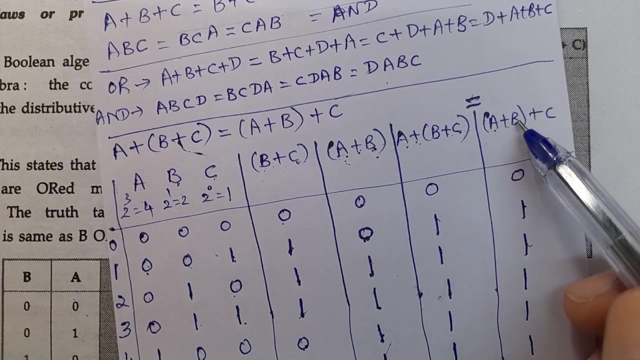 you don't want it, but I tell us, or to table. so then, a or B or with the C, a or with is the same as is the same it, not same. a or B or with the C is the same as a, or with the B or C, okay, same it all three. 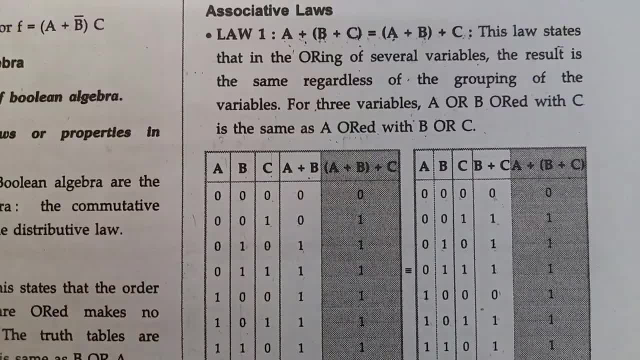 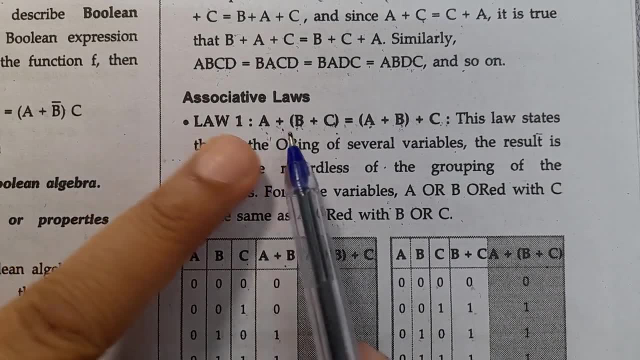 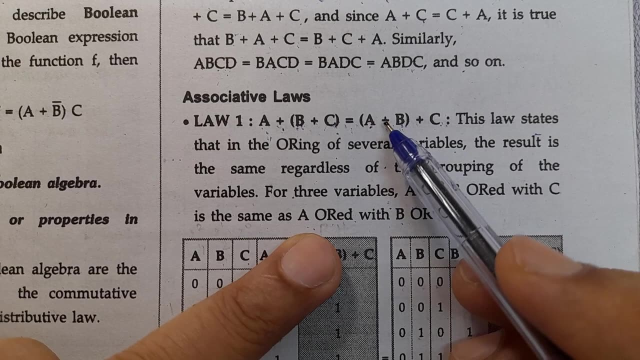 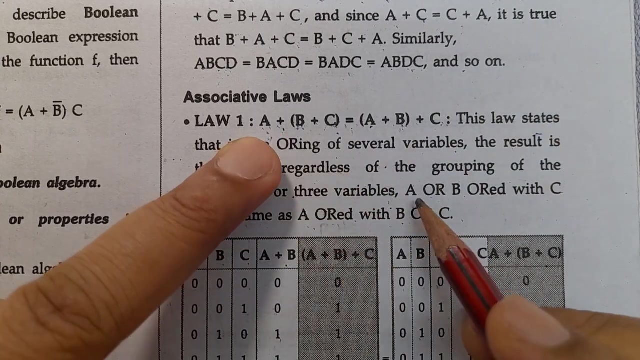 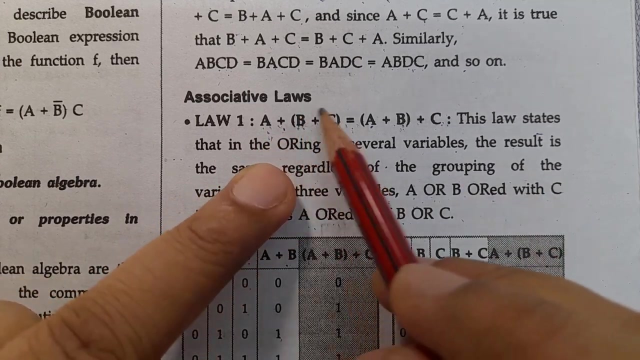 though. so the key he'll hear: odo yay, yay de la. so the key he'll hear: odo yay, yay de la. Then we have to do this Like this: Next is the same as A ORD with B. This is grouping. 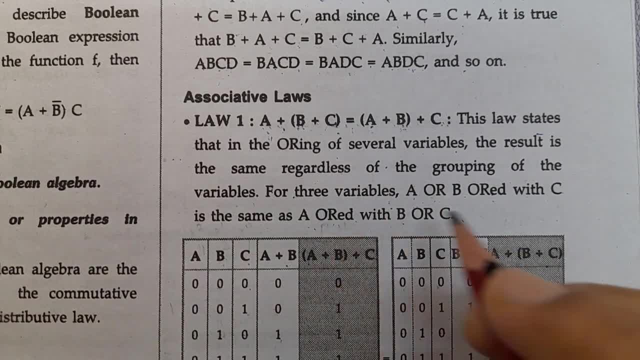 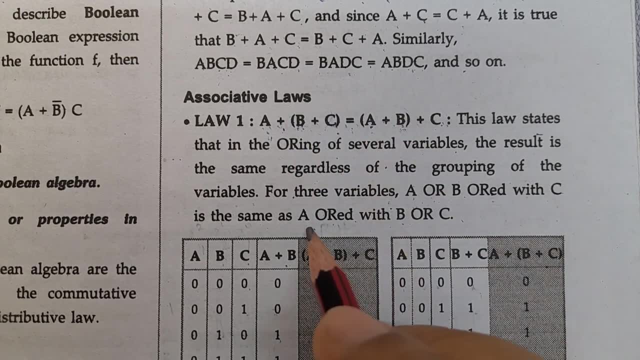 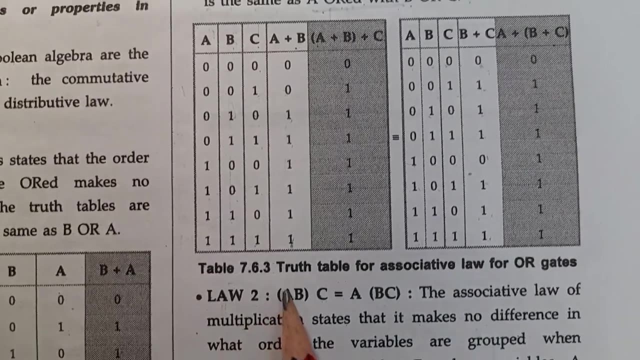 If you say ORD with, it is a group B. ORD with C, this is a group A. ORD with B, this is another group. This is grouping OR C. if you say it is a plus C, Next table 7.6.3.. 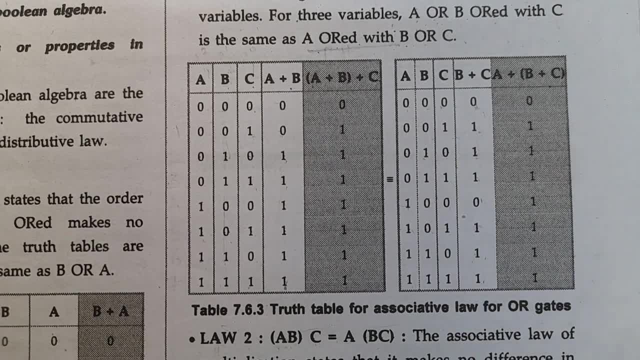 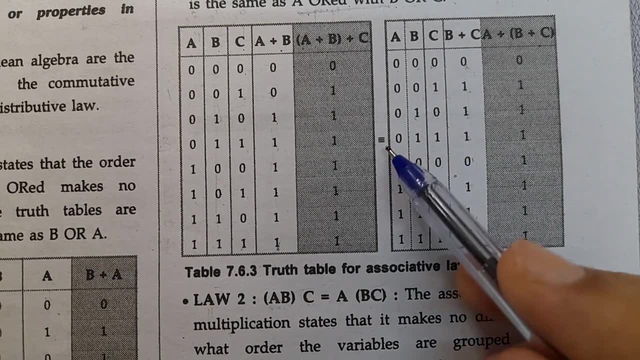 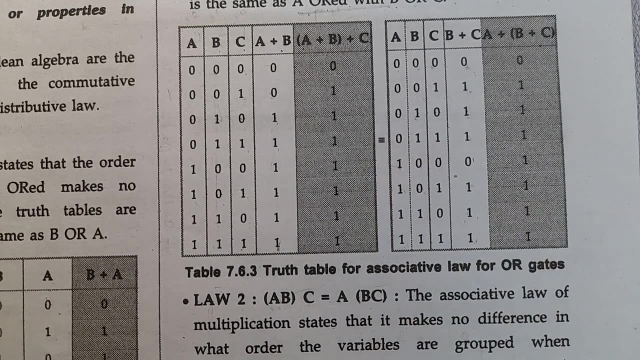 To the table for associative law for OR gates. Next here 3 equal lines have come. That means it is the same as D. There are 3 lines here, So it represents it is the same as D. Next law 2.. 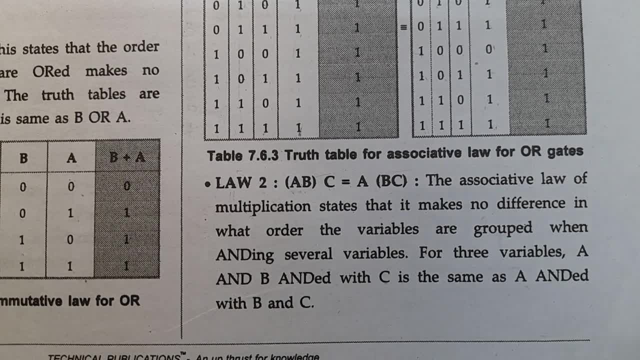 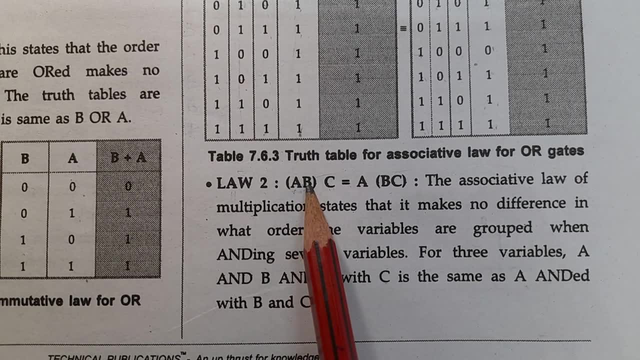 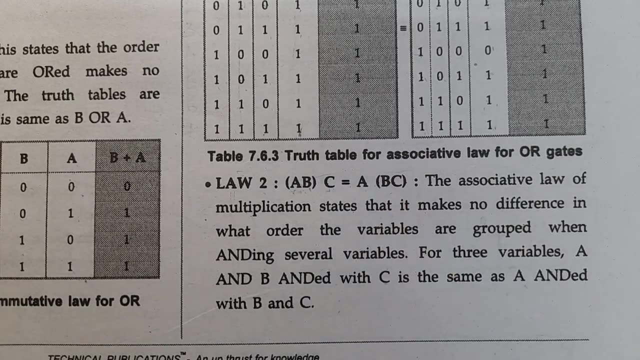 Here OR operation has happened. Next is AND operation. So in AND operation, this is the same. A ANDed with B, Okay, AND C. A AND B ANDed with C. The associative law of multiplication states that 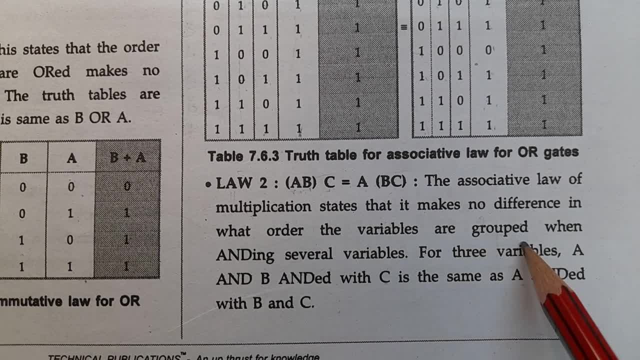 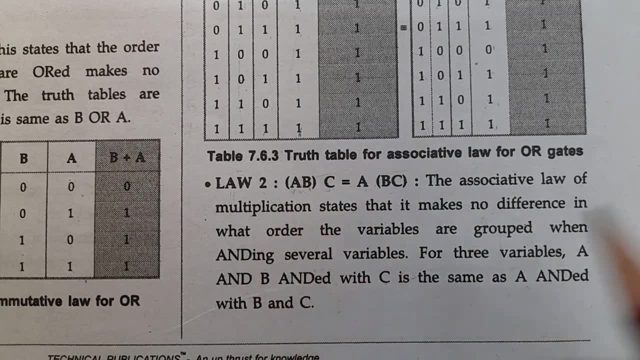 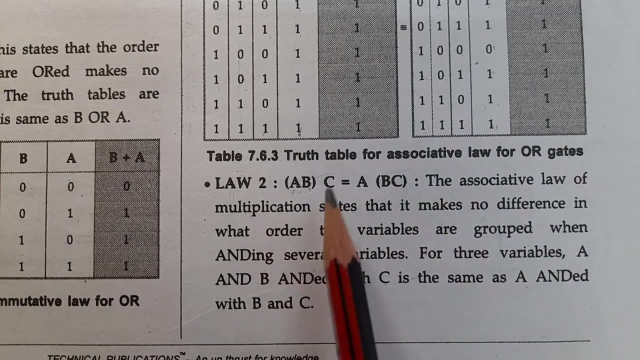 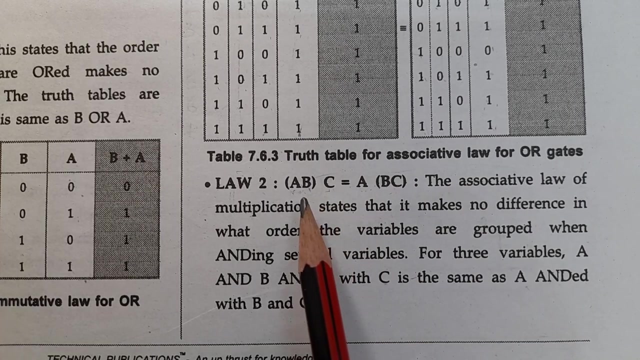 it makes no difference in what order the variables are grouped. When ANDing several variables In AND operation, how many groups were there? That means the result remains the same For 3 variables: A AND B. A and B anded with C is the same as A anded with B and C. 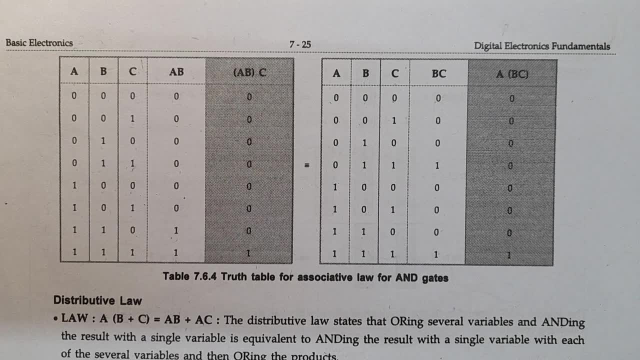 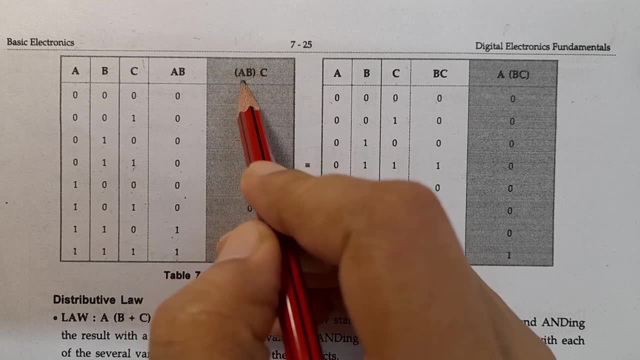 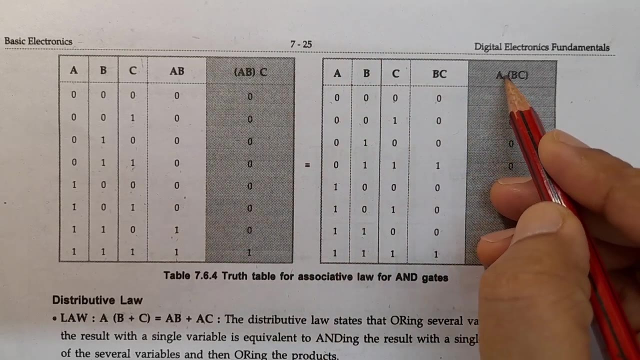 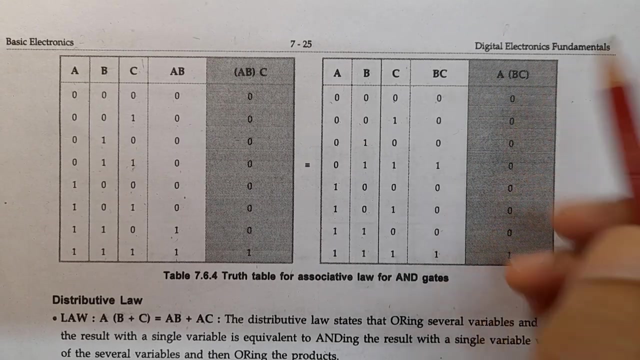 So three variables. truth table: A anded with B group is not there, so A anded with B and C. Next, here, A and B anded with C group is with. This is not and operation, so B anded with C. 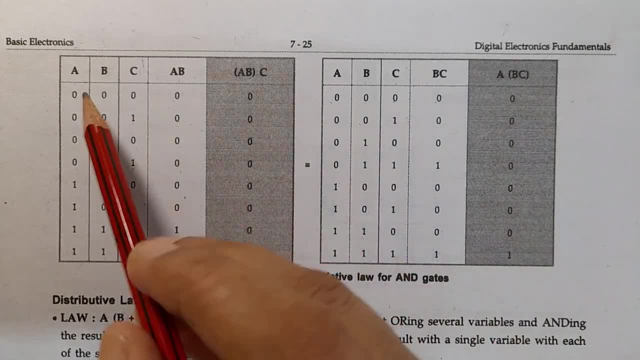 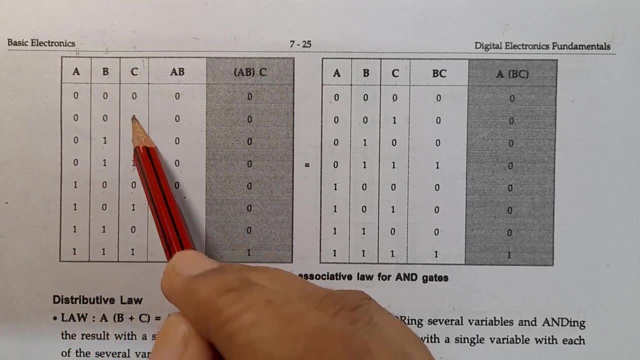 A and B anded with C is the same. So A, B, C. so here 1, 2, 4.. So 0 is 0, 1, 2, 3, 4,, 5, 6.. 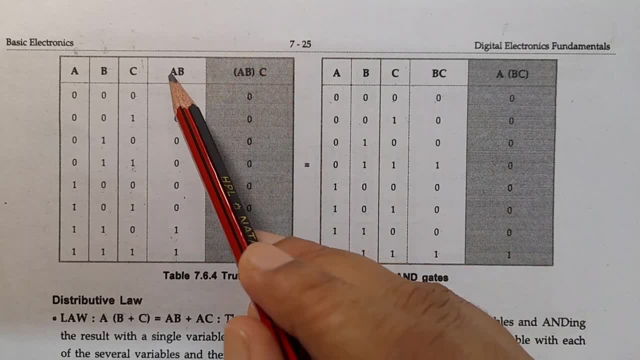 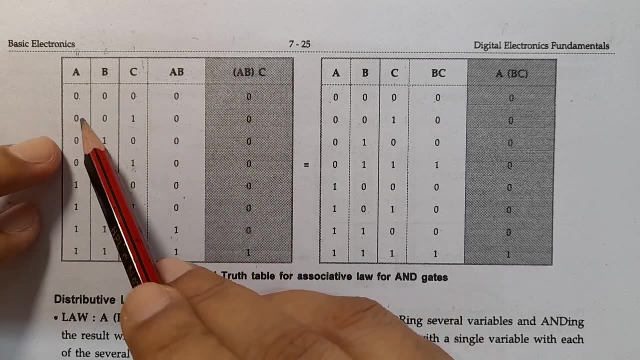 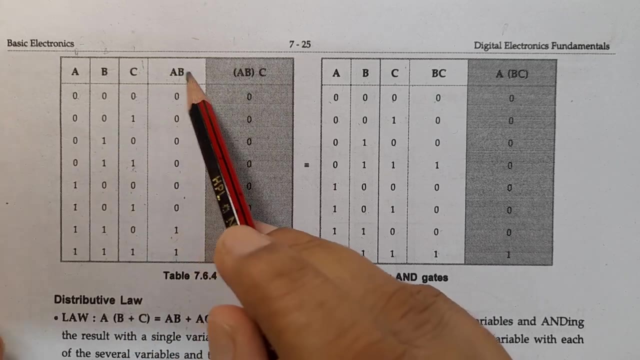 7, already. you know this much right. Ok, A anded with and B. A and B means multiply 0 into 0 is 0. If any one input is off. so A anded B is 0, off. 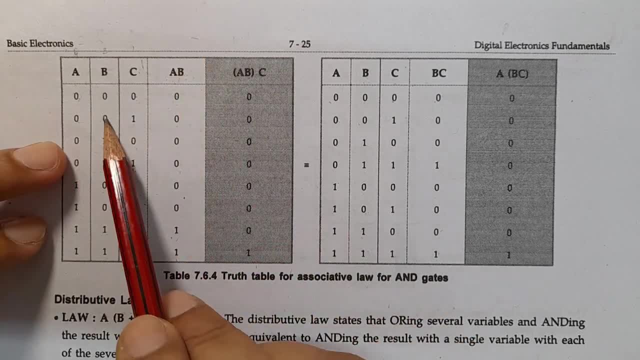 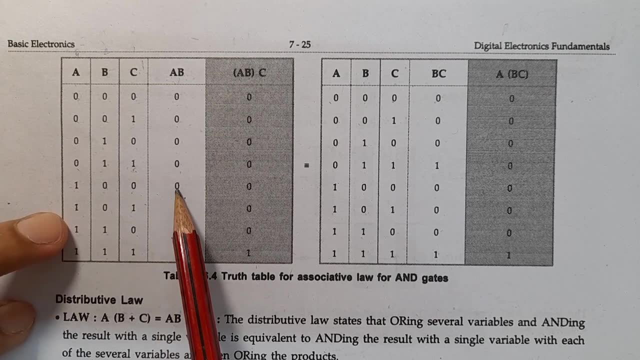 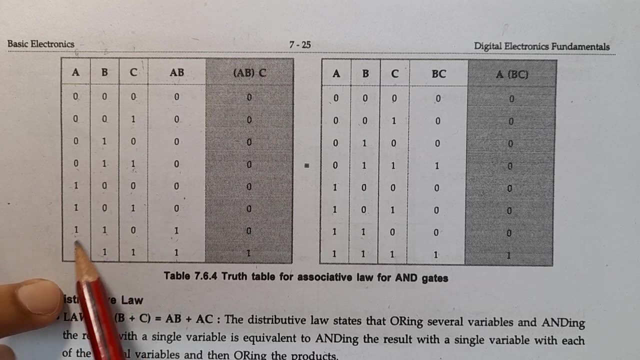 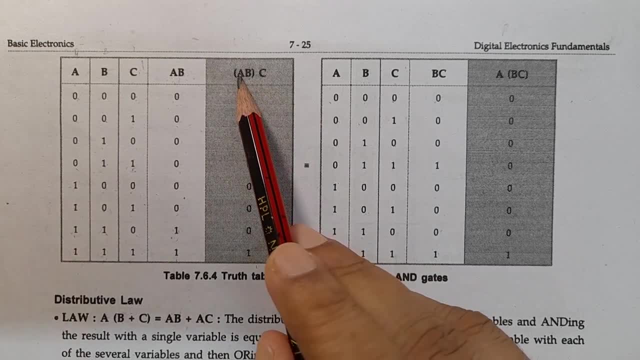 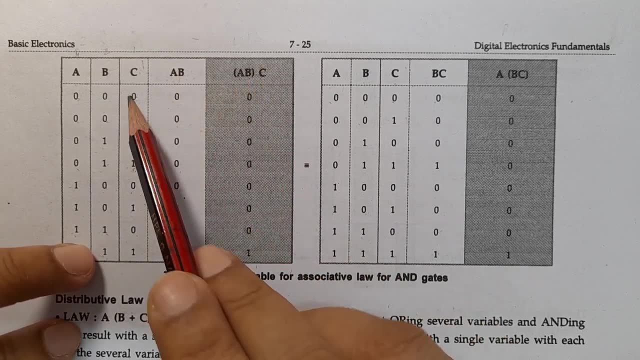 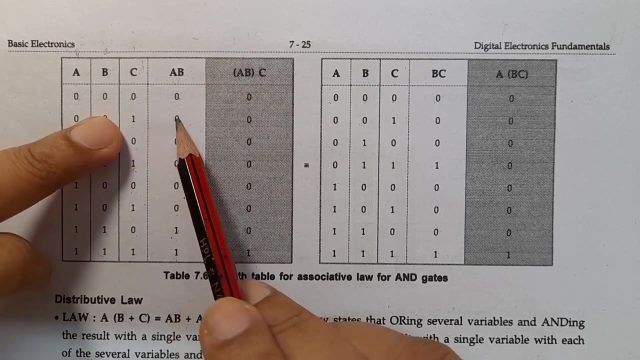 So like this, it will be off. Next, A anded with B and C. if you say like this, you have to multiply this with this: Both these switches are off, off. Here, A anded with B is off. so compare these two. this is off, this is off. 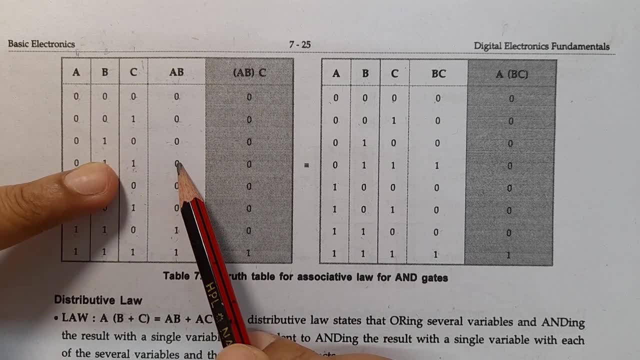 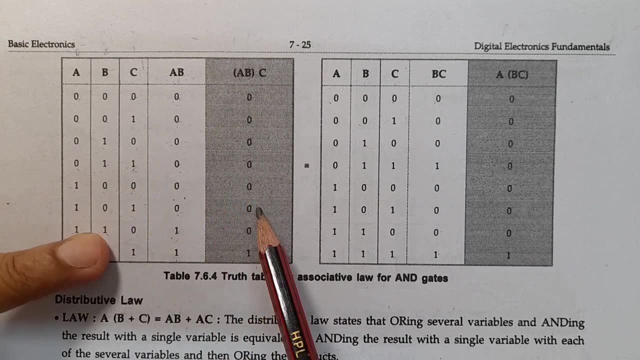 Here, A anded with B is off. so compare these two: this is off, this is off. Both these two switches are off Here. one switch is off, so off. If A, B is both off, then off Here off. 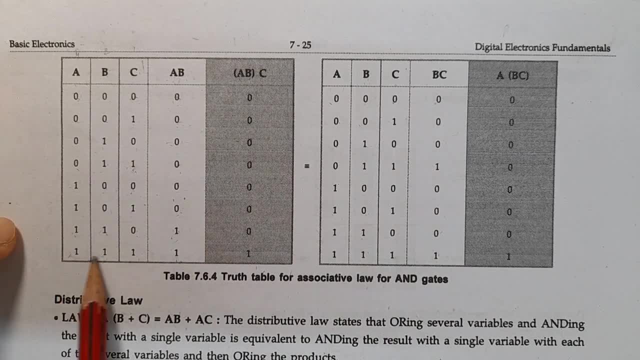 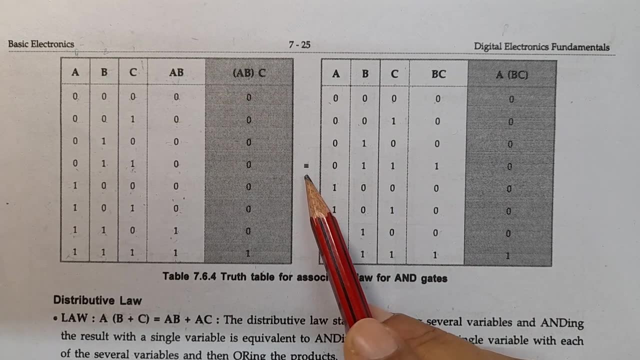 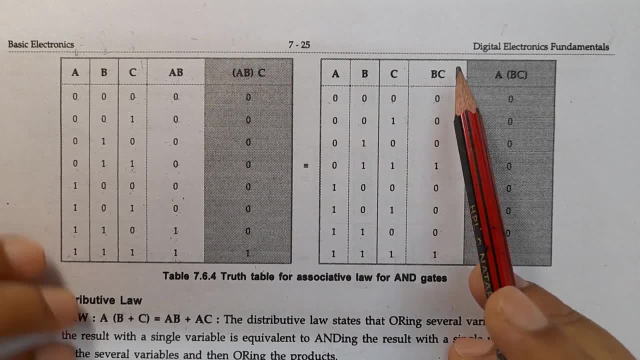 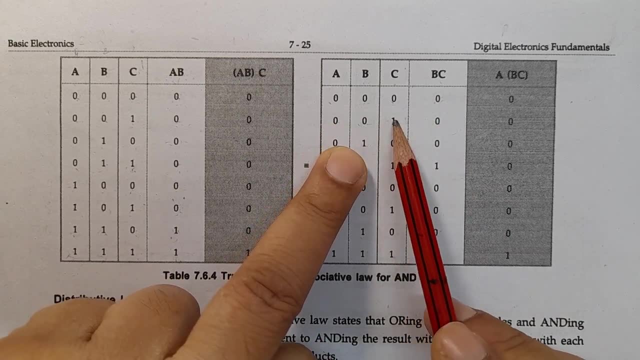 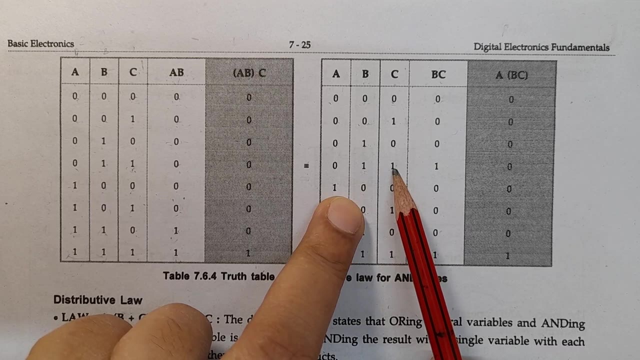 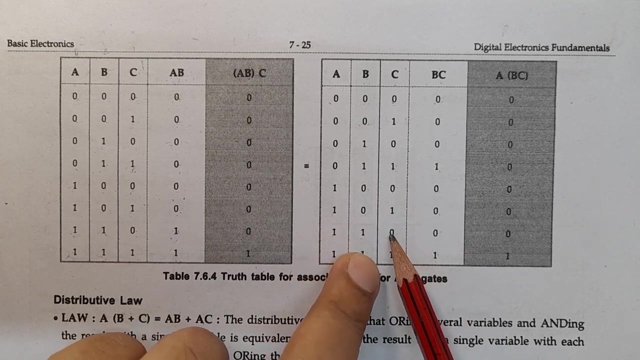 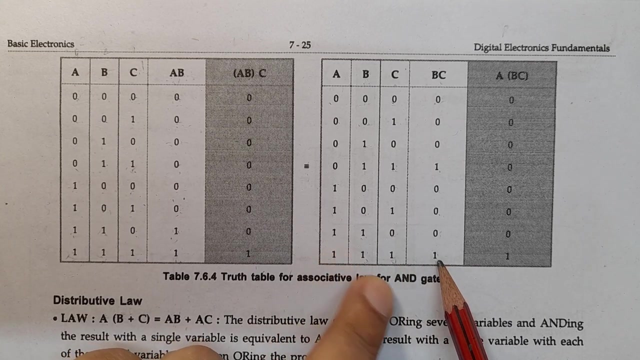 How is the same here in inputs B anded with C, C is here, See. So both the switches are off. Here B is off B and with C is 1.. So 0 into 1 is 0.. 1 into 0 is 0. So both the switches are on. So on, Both the switches are off. Here B switches off, Here C switches off. 1 into 0 is 0.. Here two switches are on, B and C. Two are on. Here it is on. 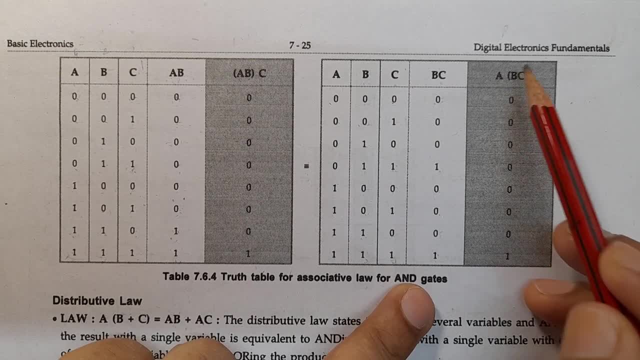 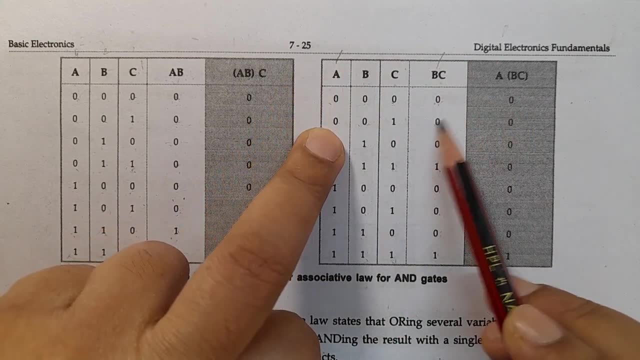 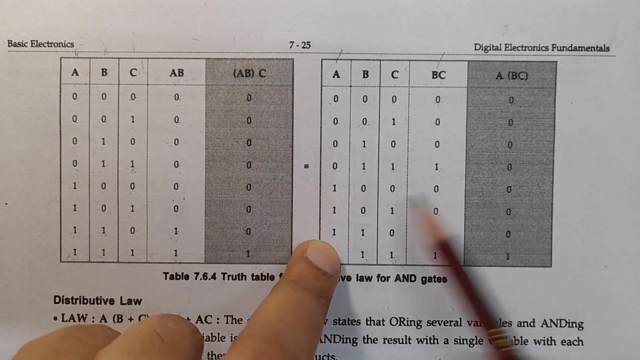 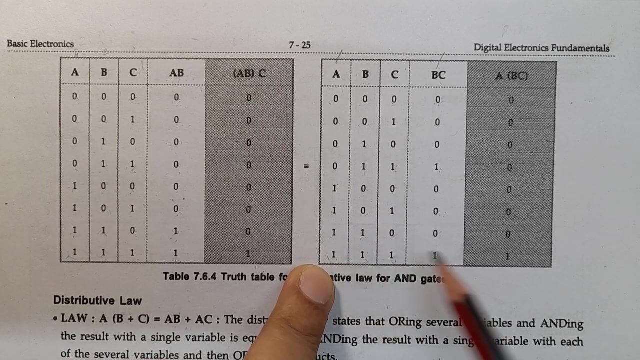 Next A and B and with C. So this and this have to be multiplied 0: 0, 0.. 0.. Ok, Two switches are off Off Here. A switches off. 0 into 1 is 0.. 1 into 0 is 0.. 1 into 0 is 0.. 1 into 0 is 0.. Both the switches are on, A and B, C. Two switches are on, So output is on. 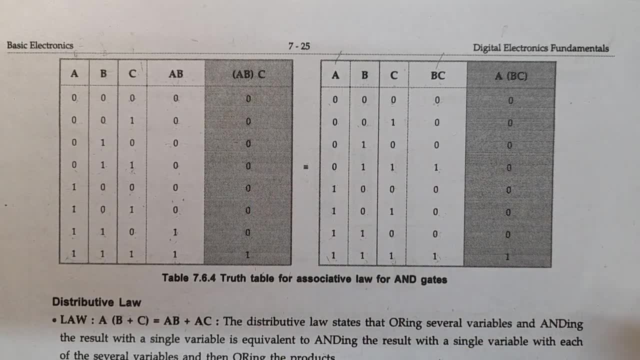 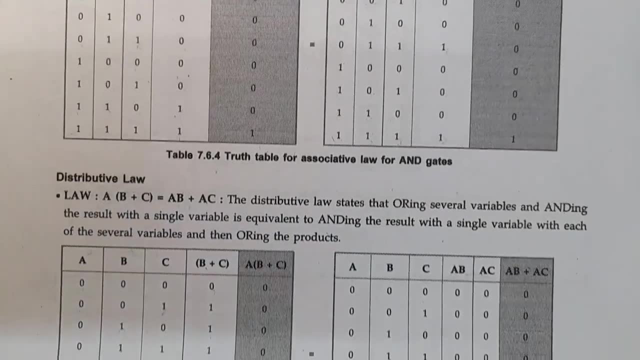 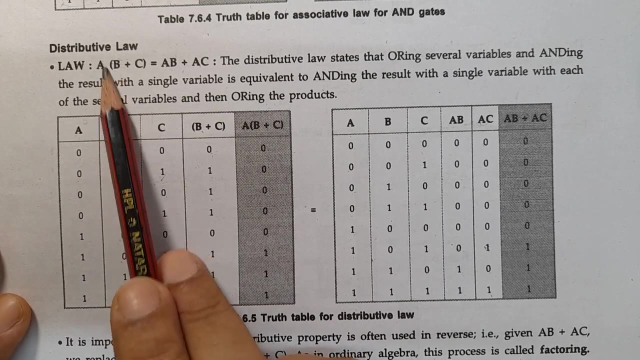 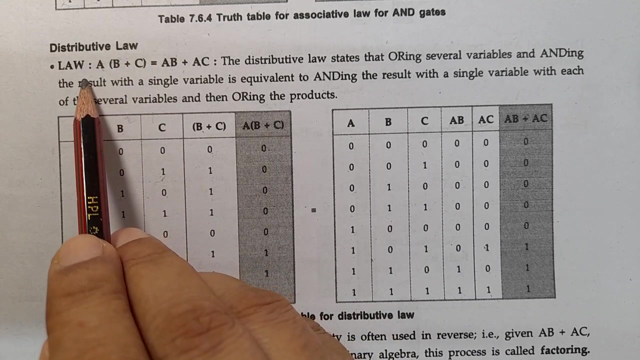 Ok, This LHS equal to 0.. RHS Table: 7.6.4.. Two table for associative law for and gates. Next last, distributive law. Ok, Distributive law in which A into B plus C, That is A and. Ok, This is A anding the result of B oring with C. 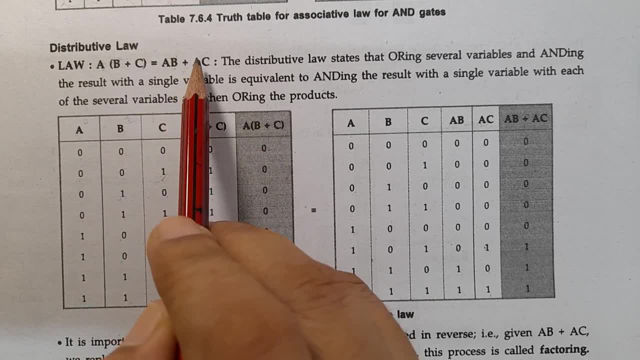 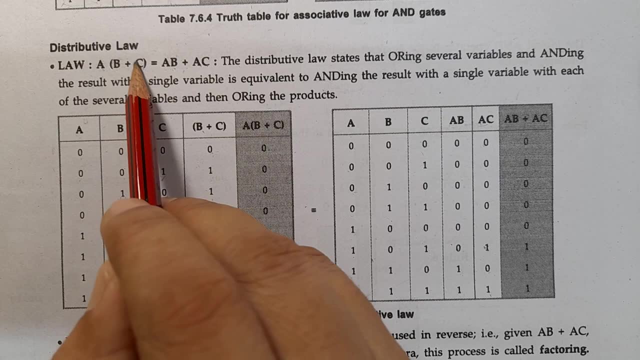 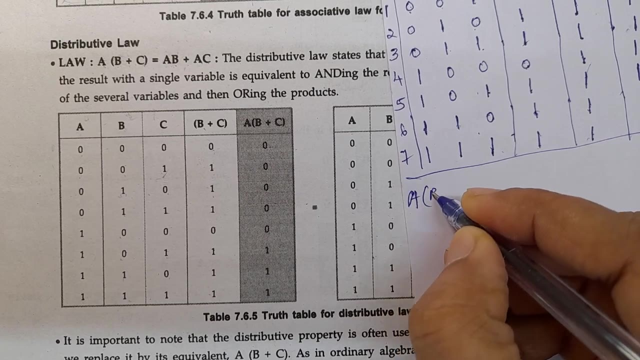 Ok, So here A and B, or with A and C, The distributive law states that oring several variables, Oring operation, Several variables, Like example: Here: A is there, Oring operation. Oring operation: Here B, C is given. 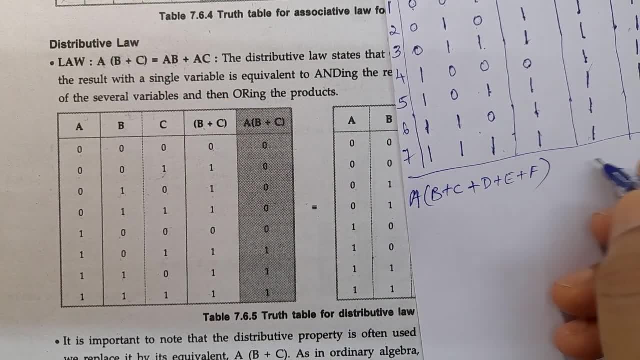 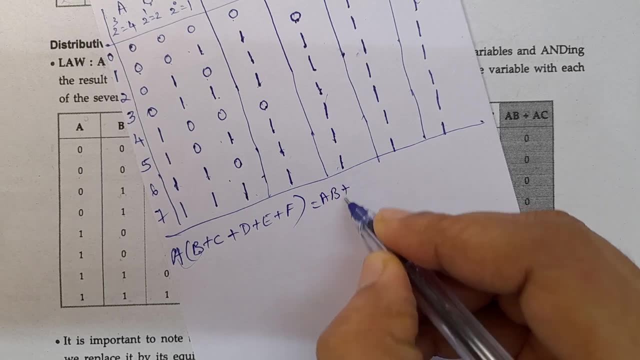 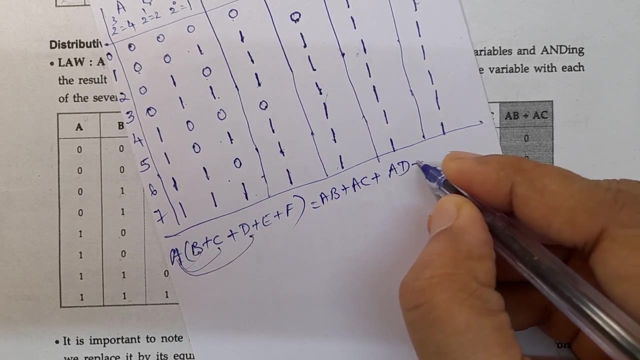 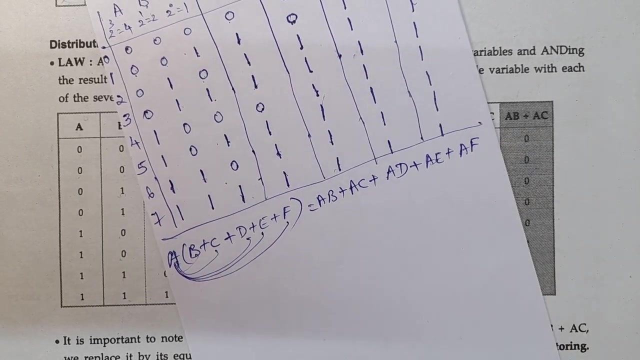 D is taken, E is taken, F is taken. Here N and RHS will come. Distributive law: A, B or A and C, or A and D, or A and E, or A and F, Like this. This is what it says. 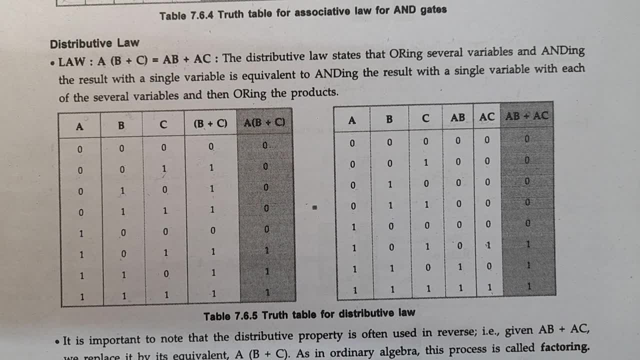 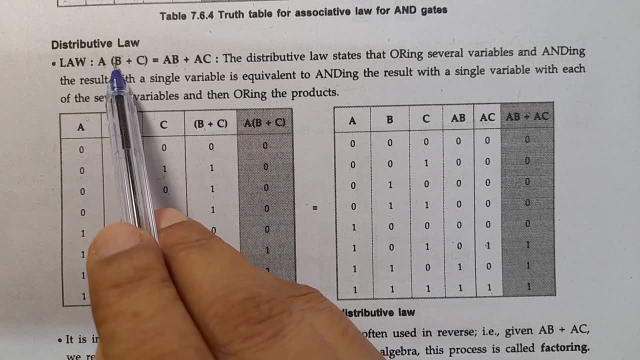 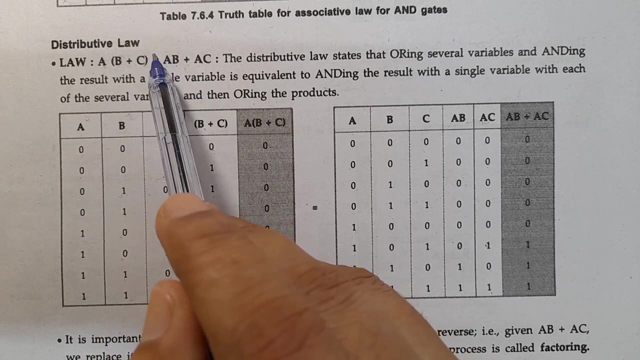 Distributive law states that oring several variables and anding the result with the single variable- This is single variable Here Variable This is all- B, C is two variables, Because several variables Oring with several variables And anding the result with a single variable is equivalent to. 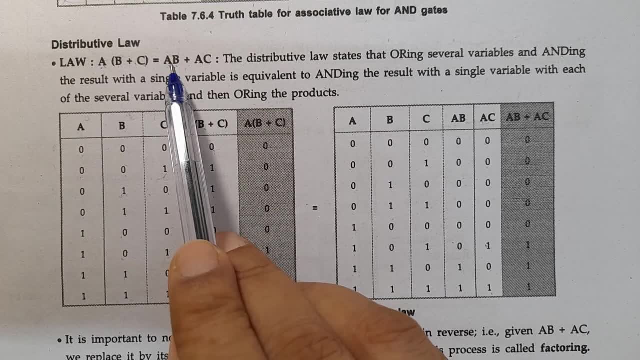 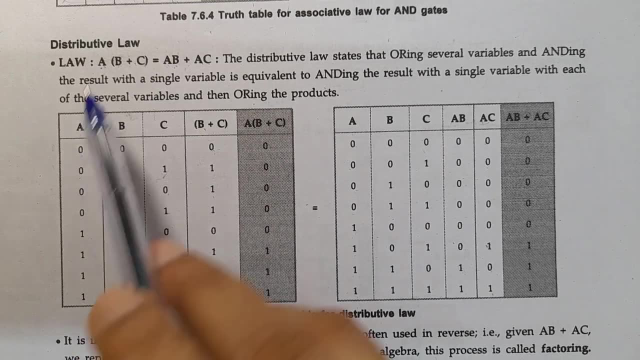 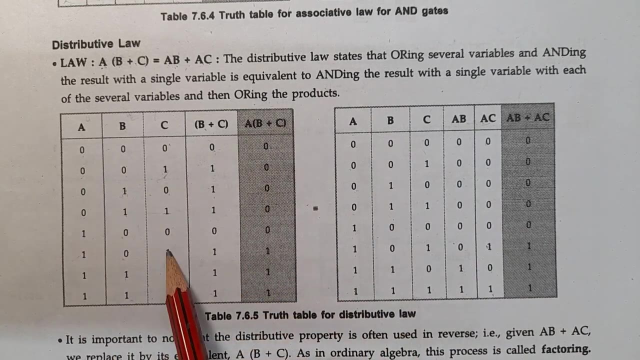 anding the result with a single variable, with each of the several variables, And then oring the products. That is it. So A, B, C input should come first, So 0, 1, 2, 3,, 4,, 5, 6.. 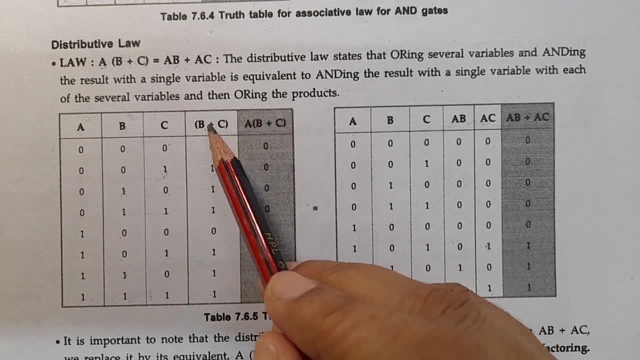 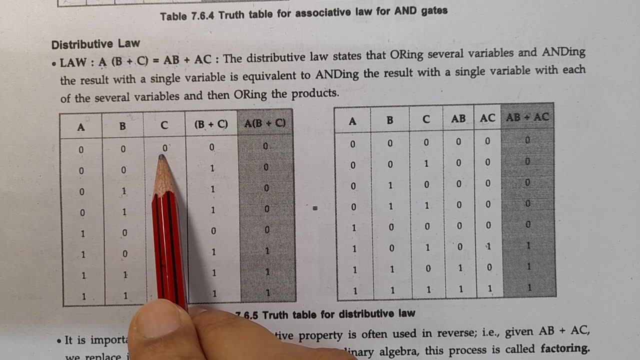 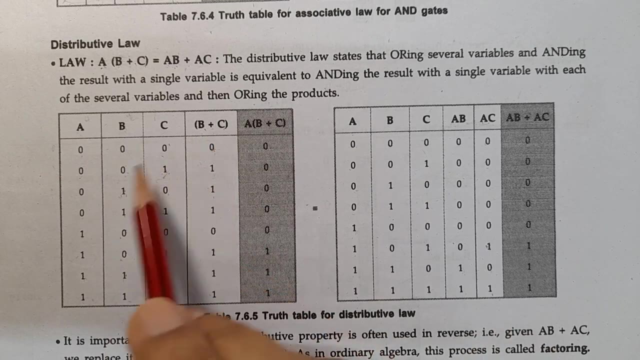 7.. This is the result. B oring with C means B ored with C. So these two operations will give us 0. Any one of them can be turned on In two inputs. any one input is turned on in the operation of oring, it will be turned on. 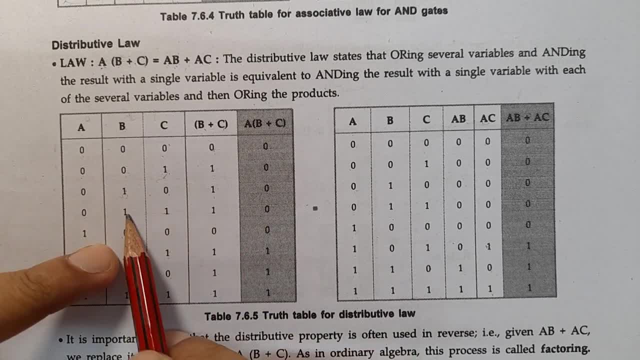 See Here: 0 plus 1 is 1.. 1 plus 0 is 1.. 1 plus 1 is 1.. Both the switches are off. Turn it off Here. one switch is turned on, See, It will turn on. 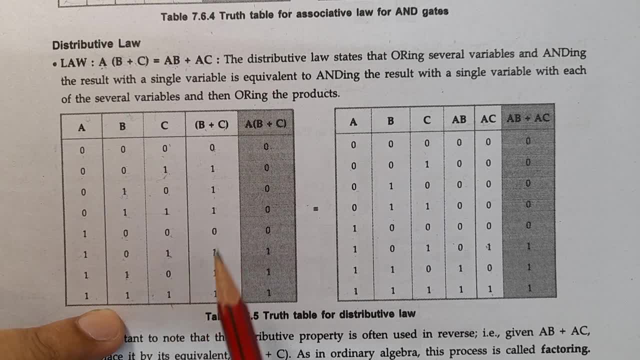 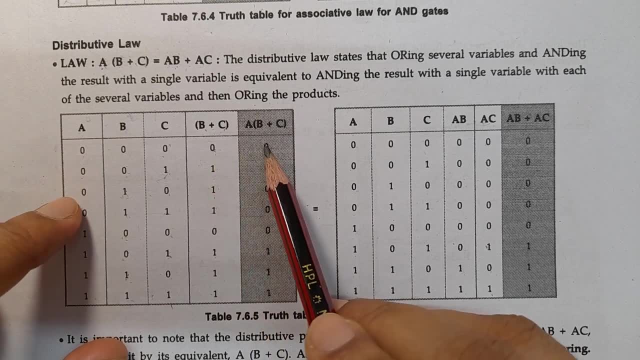 This is turned on. It will turn on Here. two switches are turned on. It is turned on. Now we need to do the AND operation, That is, we need to multiply: 0 into 0 is 0.. 0 into 1 is 0.. 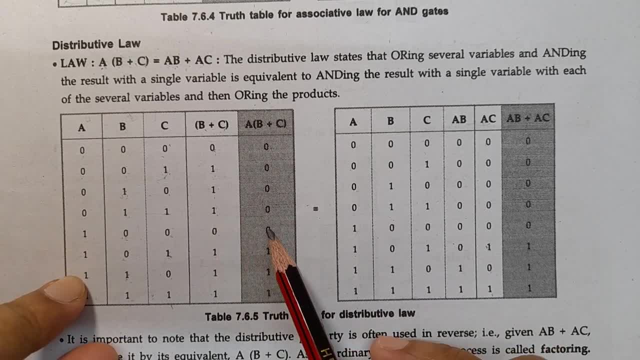 0 into 1 is 0.. 0 into 1 is 0.. 1 into 0 is 0.. 1 into 1 is 1.. 1 into 1 is 1.. 1 into 1 is 1.. 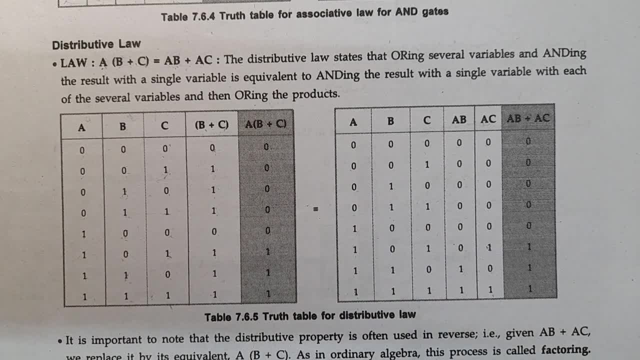 That is, if both the switches are turned on. only then the output will turn on. That is the AND operation. Any one switch is turned on, that is the OR operation. That's it. So now we need to do the AND operation. 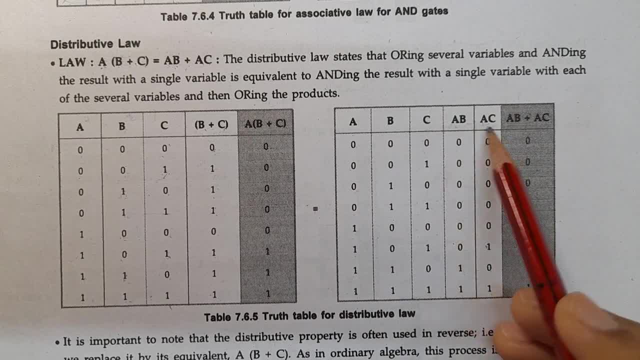 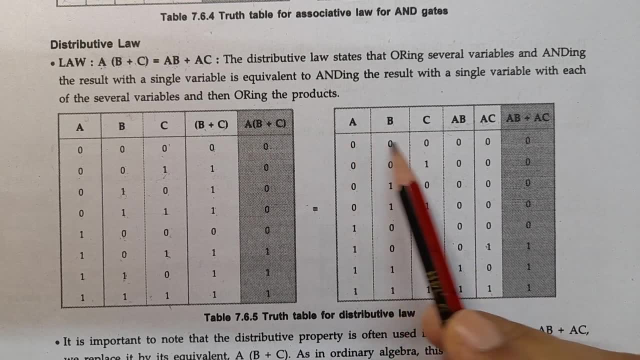 This is the same as here. First A: This is not distributed. This is RHS, This is LHS. This is for RHS. First A B. We need to do A and B, So both the here, both are off. 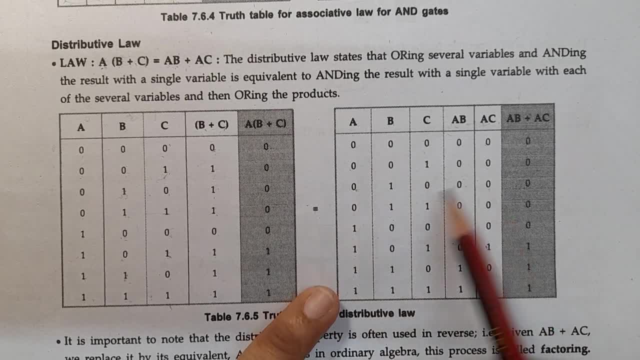 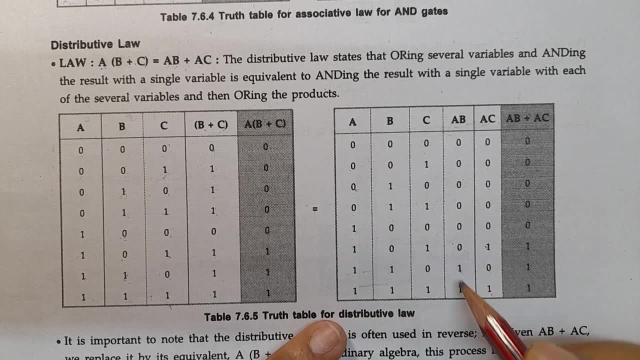 Here one switch is turned off. The OFF is 0.. Only if 2 switches are turned on it turns on. Only in these two cases it is turned on. So like this: A and B are turned on here, Rest are 0..